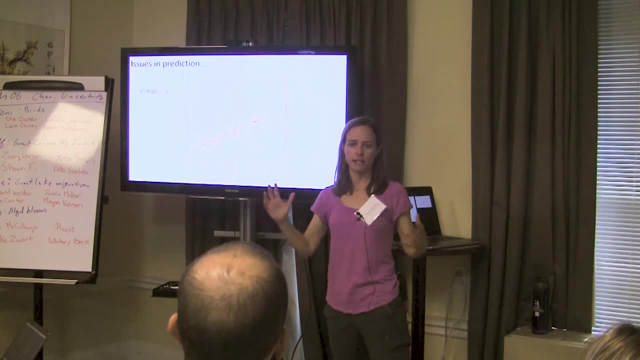 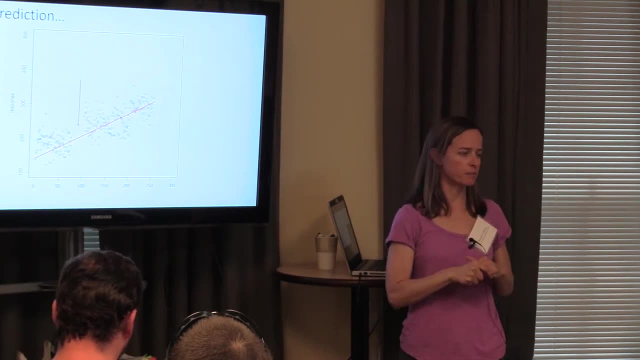 you're fitting some linear model through a cloud of data and sometimes those data are missing, and what do you do when they're missing? You guys have now all done confidence intervals and predictive intervals, and so you know that. you know you come out with 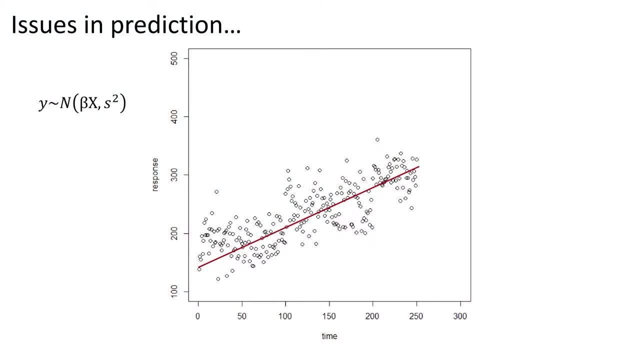 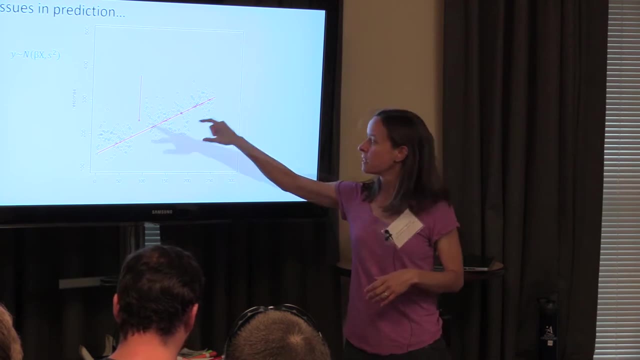 confidence intervals that are based on how tightly you got those parameter values, the precision of the parameter values right, And you can always make those confidence intervals smaller by adding more data in. You get better parameter value estimation. but when you do your predictive interval you want to include some of that uncertainty because you're predicting. 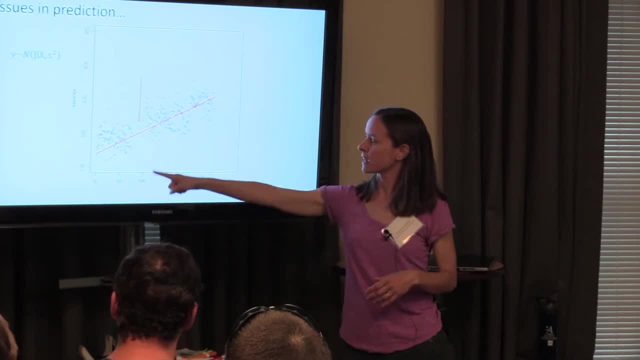 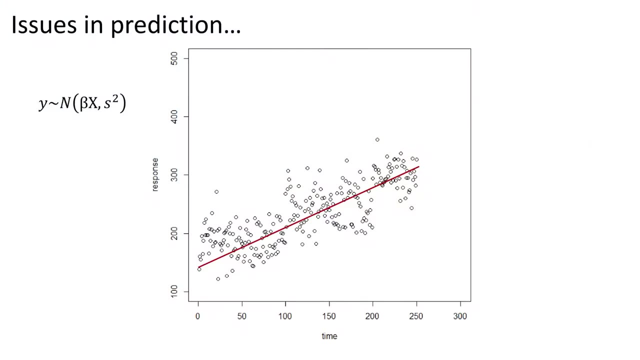 so if you're predicting at a given spot here on the x-axis, you would start with the mean, right. So your prediction would be at the mean, but you would have some interval around it based on both of those. Okay, Okay. 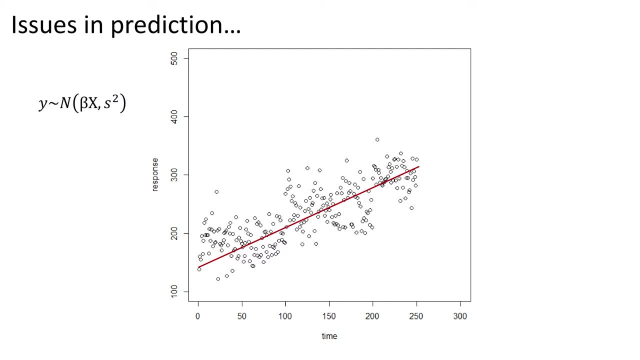 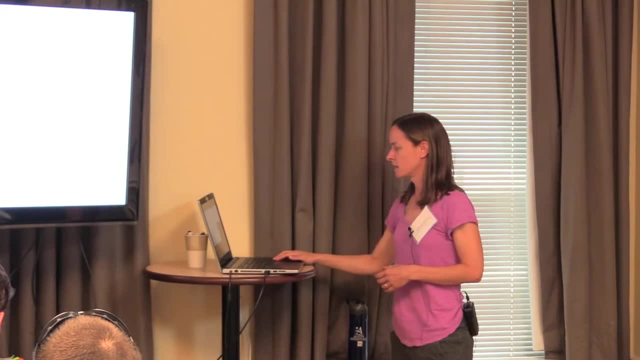 Okay, So you can imagine both that observation error and how well you were able to characterize the model. Okay, so this is kind of all background, what we've done the last couple days. And when we're forecasting we're generally thinking out beyond the end of when we have data. so 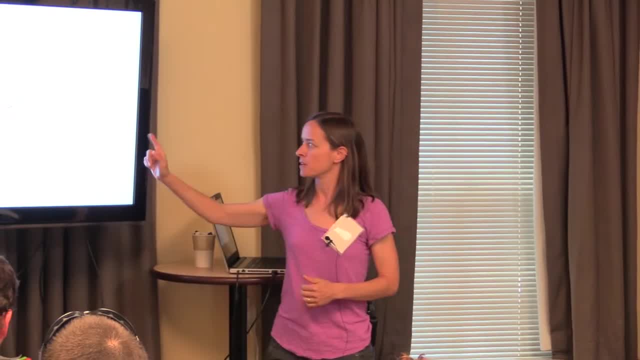 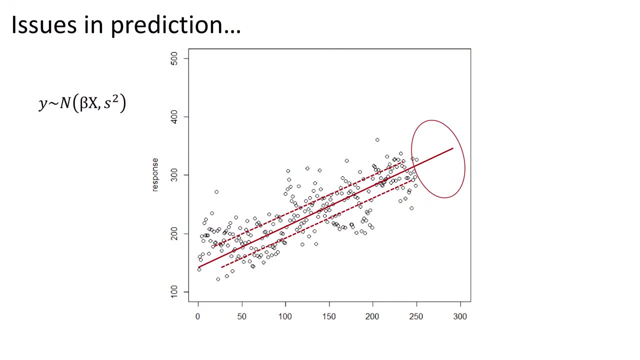 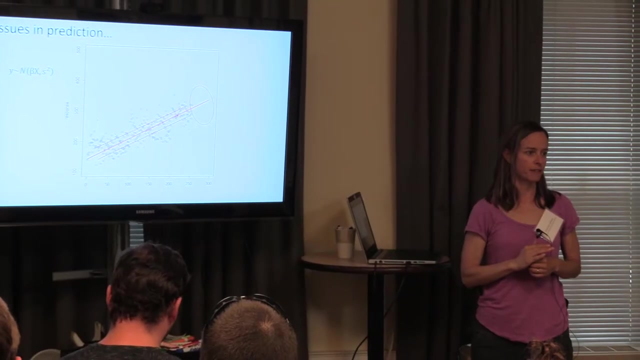 out of the range of the data that we have, And so you can imagine that the confidence intervals, and certainly the predictive intervals, get bigger. when you don't have data- and that's again a standard approach- You fit a line and you can predict out. you assume that that line is representing a bigger. 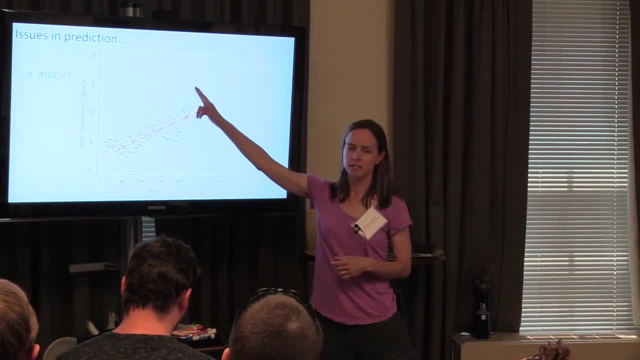 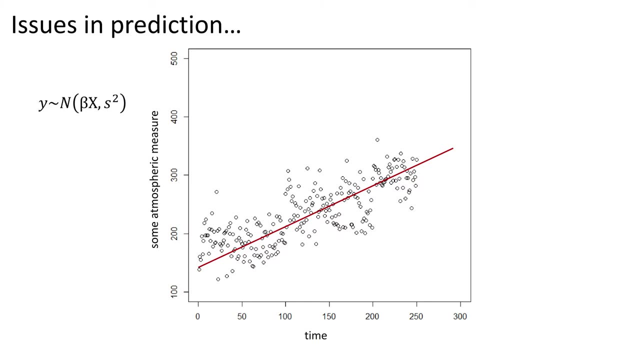 population than what you sampled. So if this is like some atmospheric measure and this is time, then if we extended the types of inference that we've been talking about, where you fit a linear model through a cloud of data and you try to predict out in time, you 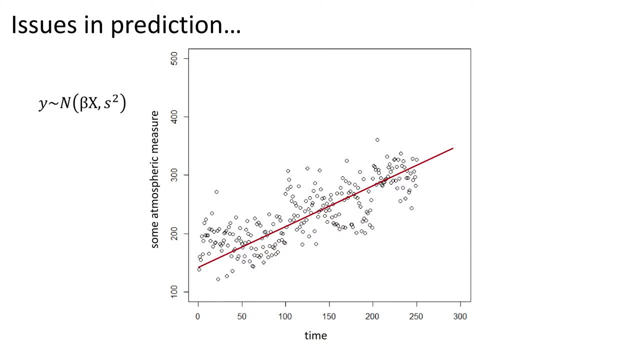 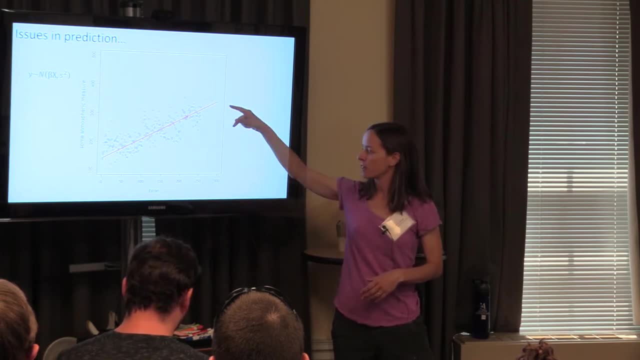 can imagine that the things that we've talked about, the reasons that you have uncertainty in the data, all come into play at once. right Like so. we're outside of the range of our. we still have observation error and oftentimes, certainly with climate or with 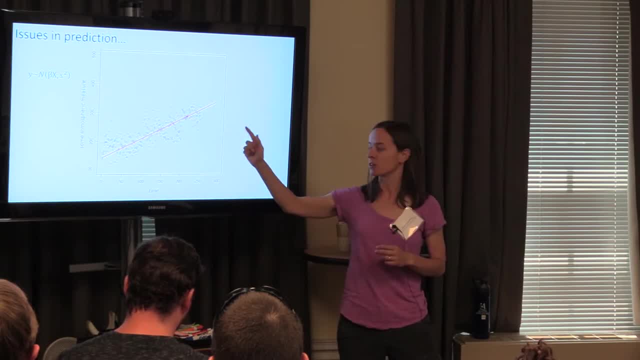 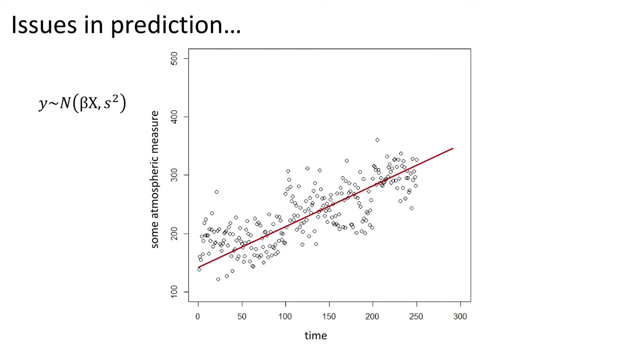 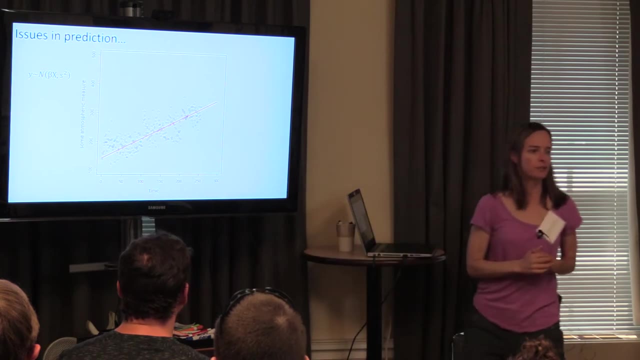 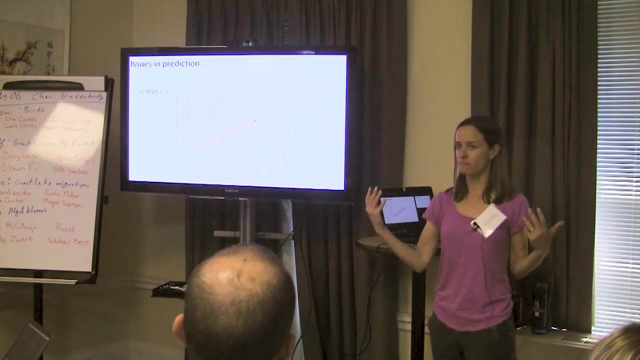 a lot of ecological things. we're also making predictions based on variables that themselves that aren't perfect. they haven't been measured completely, and maybe this, this atmospheric measure, is actually a compilation of multiple measures, and so all of that makes makes this prediction issue difficult. Ecologists have not had a ton of success in making forecasts or predictions that. 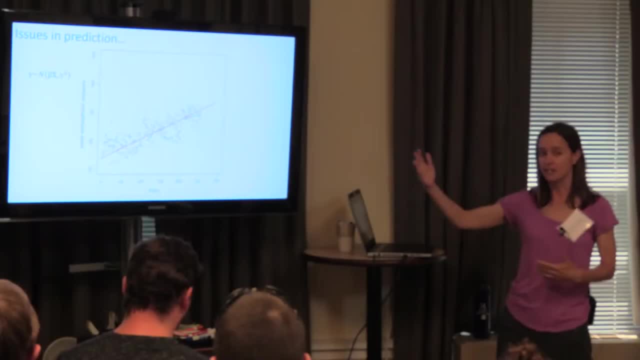 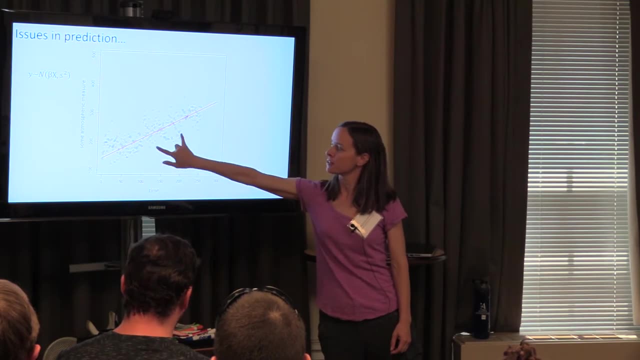 are then validated in five to ten years. even when you do wait five to ten years- and a lot of it, you know if you predict on this mean line, even if you predict within your data range, you're almost never right. if you were to make a prediction on the line and then go back and collect data, you know you don't. 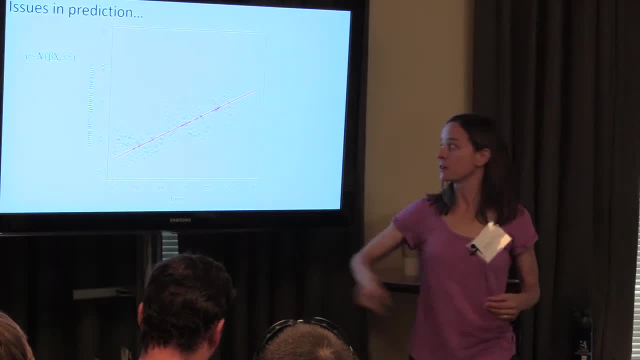 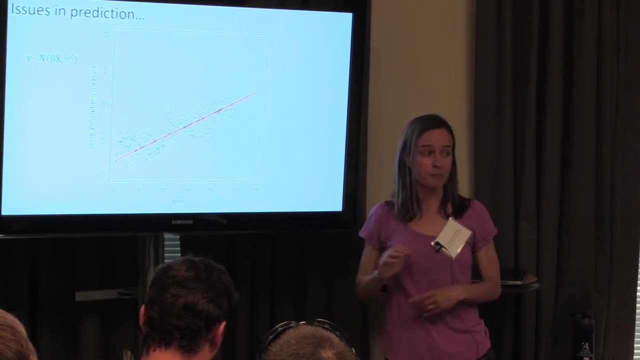 necessarily expect to get within. you don't expect to hit the line. In fact, you almost never expect to hit the line right, And so understanding how off the line and why you might not be on the line is super important, and it only gets more important when you're trying to do it outside of the range of your data. 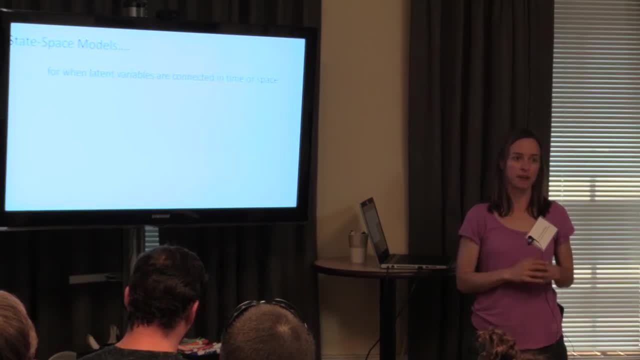 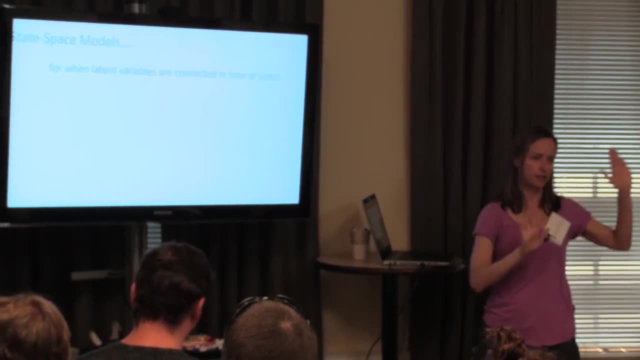 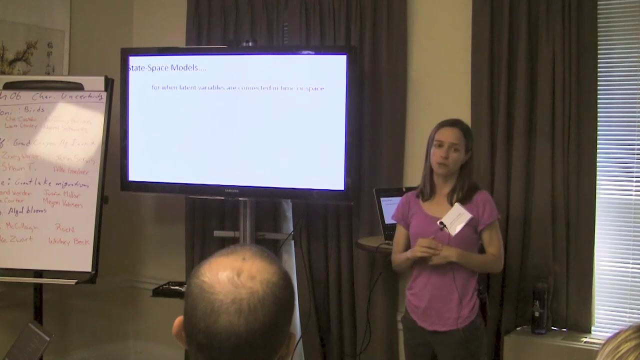 When you have a bunch of latent variables. so again you're measuring something like MPP and yet you're really measuring something else, but you're interpreting it as MPP and you have them connected in time. so you want to know how that ecosystem measure changes over. 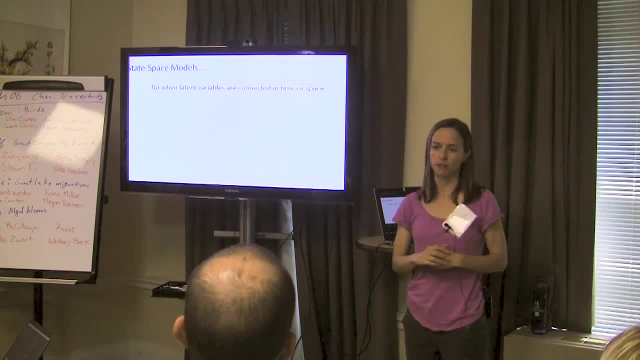 time. then you start to get into the realm of state-space models, right? So one thing I didn't point out in the last figure is I put time on the x-axis and then showed you a linear model that obviously violates the idea of independence. You could just jam all that into correlations in the 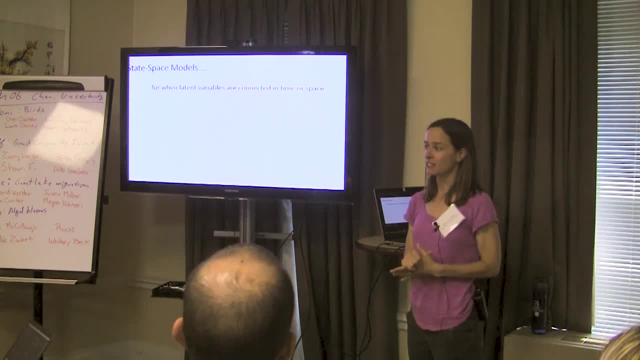 air, but that's not necessarily going to help. if you're forecasting right, It may help you get a better p-value, but it's not necessarily going to help. if you're forecasting right, It may help you get a better p-value. 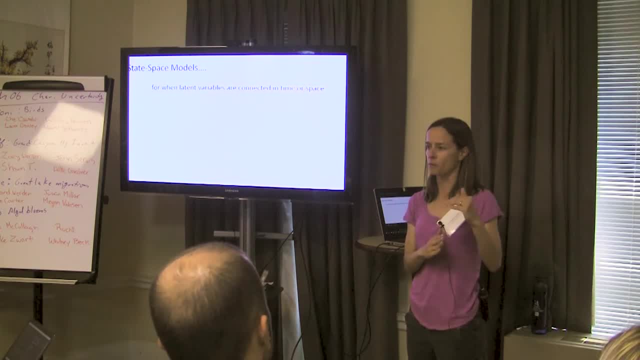 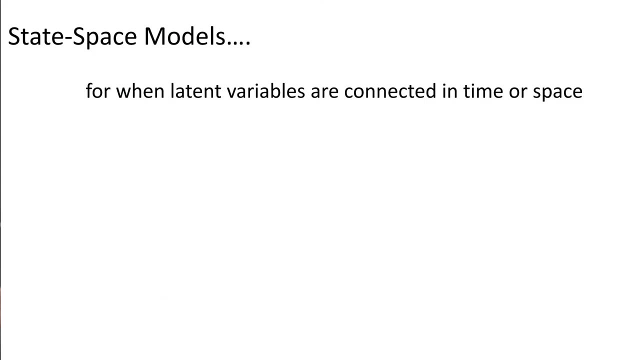 but it's not necessarily going to help if you're forecasting right. It may help you get a better p-value estimate or be more confident about your p-value on the slope, but it's not necessarily going to help you forecast outside of your data better. So when you have latent variables that are connected, 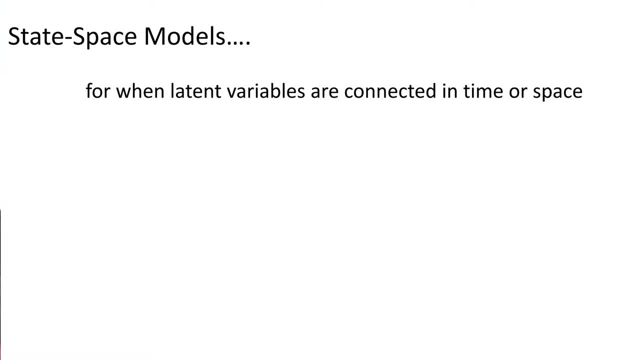 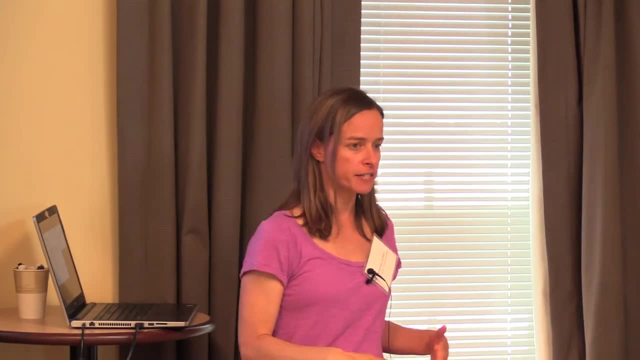 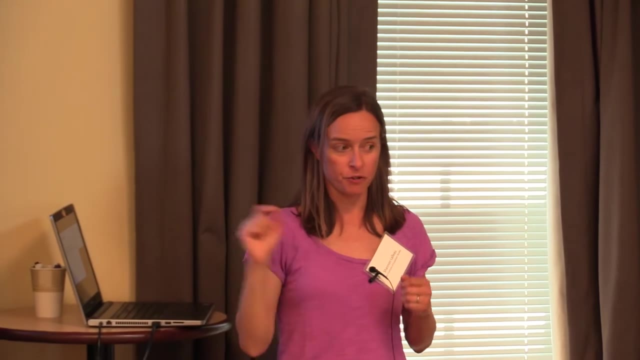 in time or space, that is, they're not independent. a state-space model is also a dynamic model, so it's a model that a future state depends on the current state or- and in much of what we're going to talk about, it's going to depend. the future state is going to be the 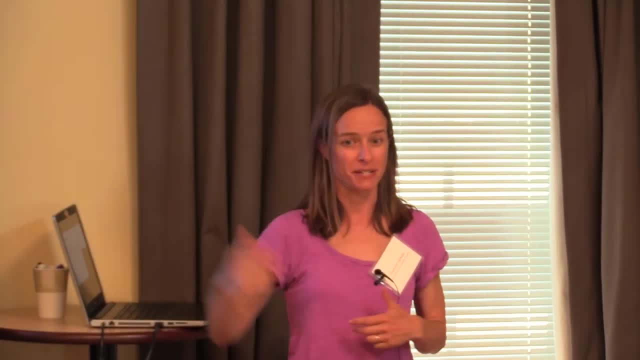 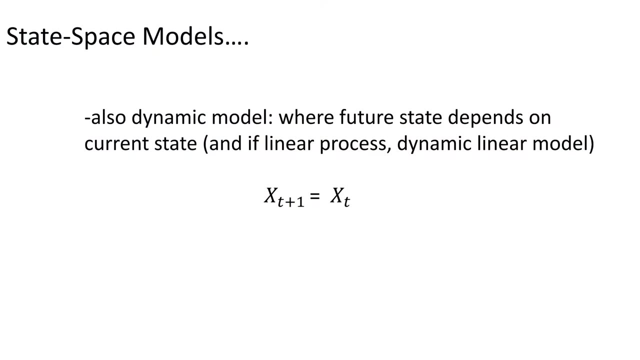 next one, right? So with just a lag of one, but it could also be different lags. If it's a linear process that you're thinking about, then it's also called a dynamic linear model. So I'm putting all this up there because you might hear some of these in ways that seem kind of interchangeable. 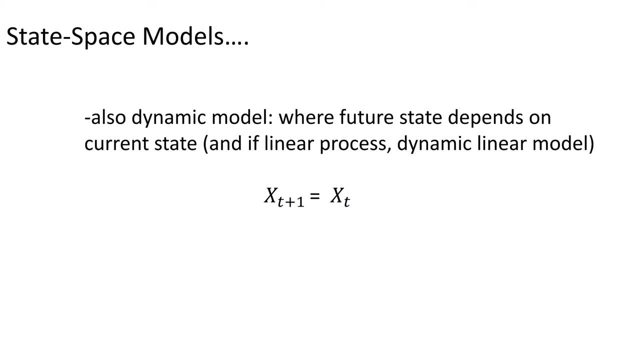 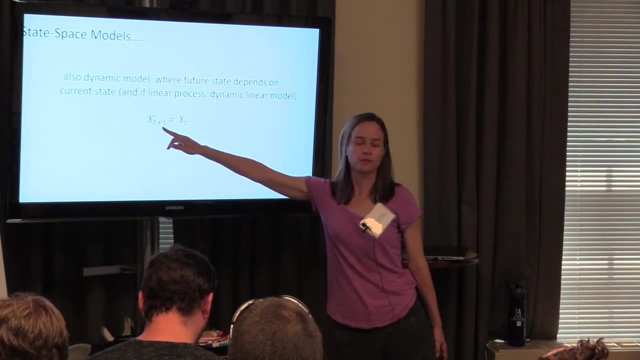 and they often are. but the dynamic model is a state-space model and if it's got a linear process, then dynamic linear model. So when I say that the current state right x of t depends on the current state, in this case would be t plus one, depends on the last. 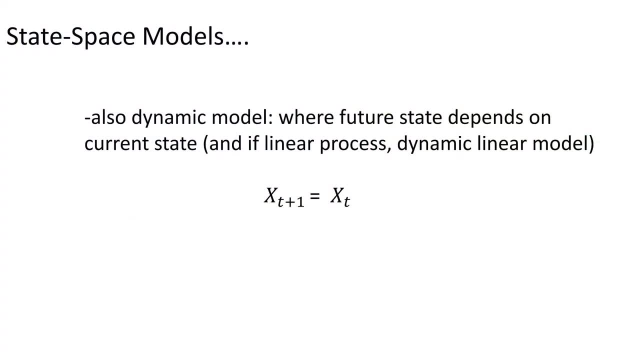 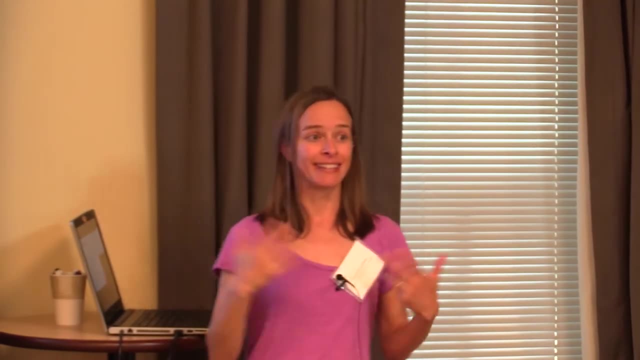 state. So knowing something about what happened tells you about what it should be now. State in this vocabulary world is the variable of interest, right, the state of the system. And if you remember, three slides ago I said it was latent variables connected. 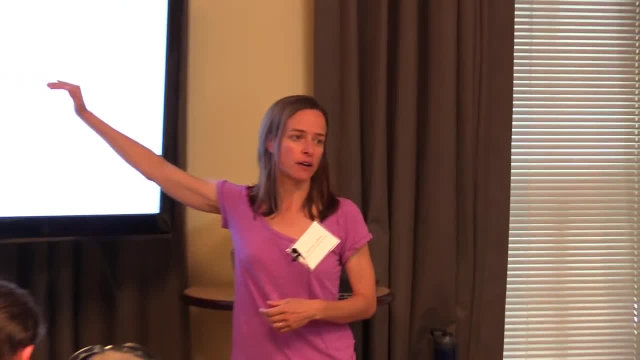 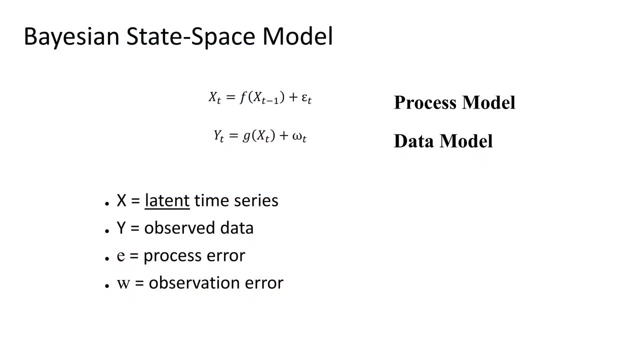 right. So the other part of this is that you have that data model. We're out there, historically latteating our data with m and m through y and then interpreting x, right, so you have your process model, which is the f, which is the x's. so so now we have moved from 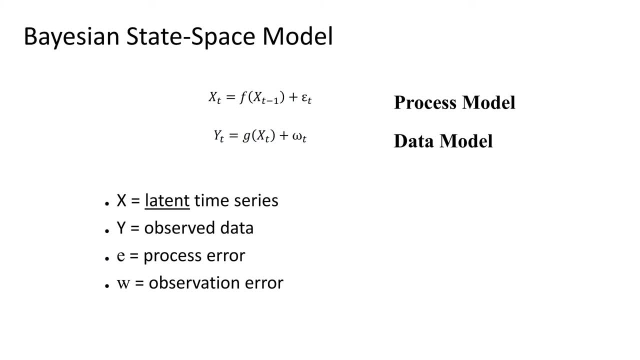 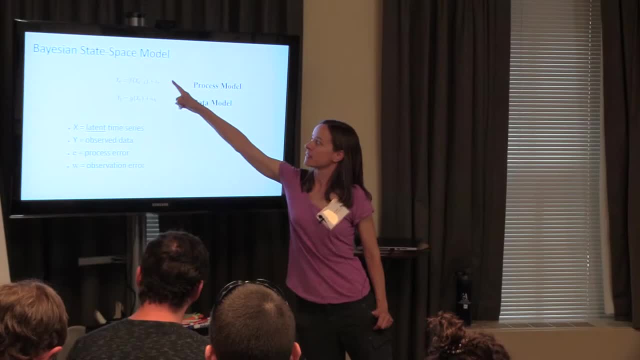 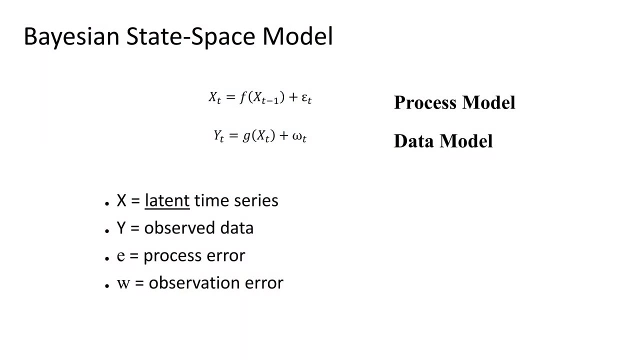 x's, as always, representing your predictor variable. okay, It is now a latent variable of interest, your response variable, but not the one you measured. and in this case, to show that minerally structure, one state depends on the last. but your observations Y are still your. 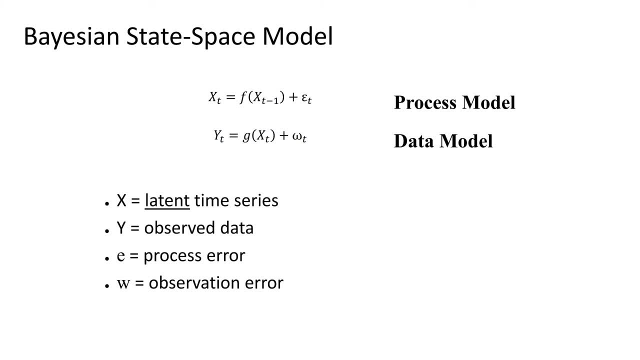 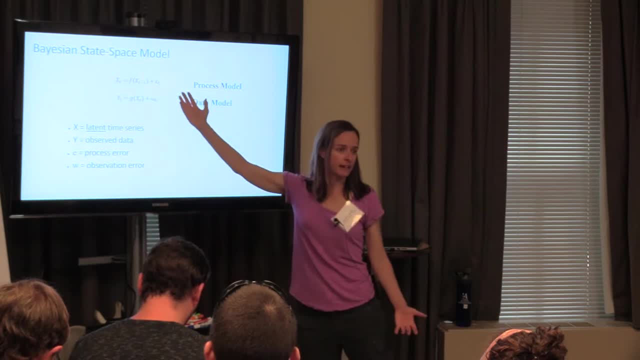 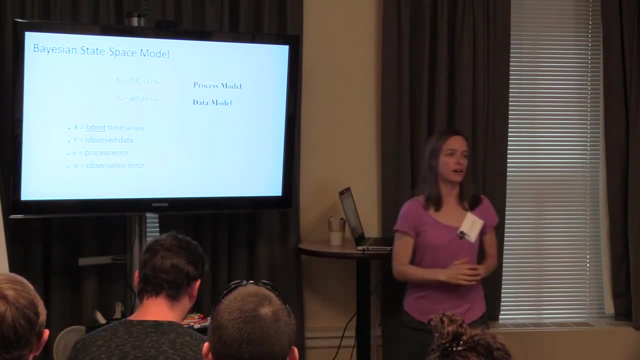 data model. they're what you measure and then you put a model in there to identify how they relate to X and, importantly, you get process error and an observation error right, so you can partition the error out and and- because this is going to be a Bayesian process, you then have distributions on those. 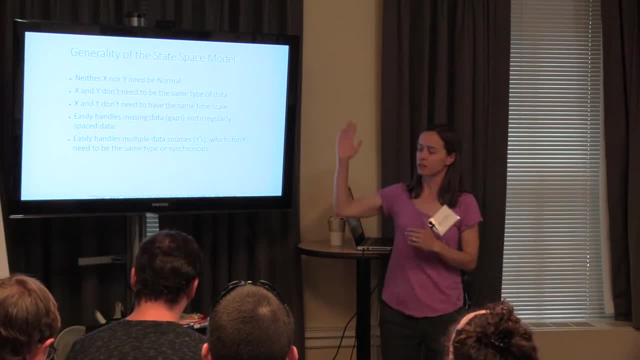 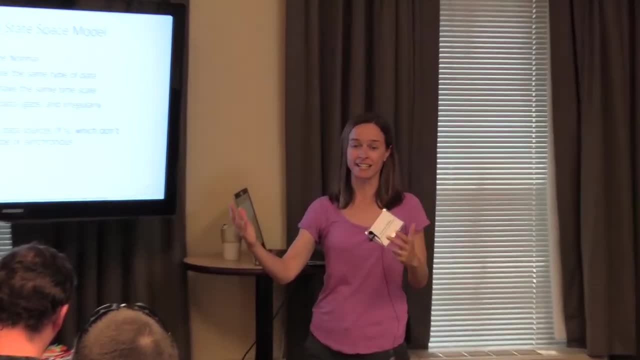 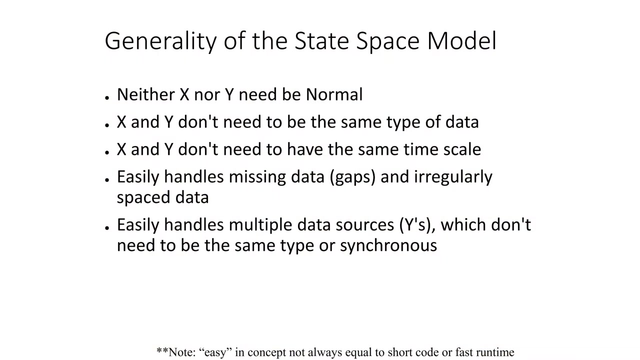 errors that that you're going to estimate. so the state space model is really. it's just a really flexible framework for identifying how states of interest transition through time or space. they don't need to be normal. neither X nor Y needs to be normal. they don't need to be the same type of data. 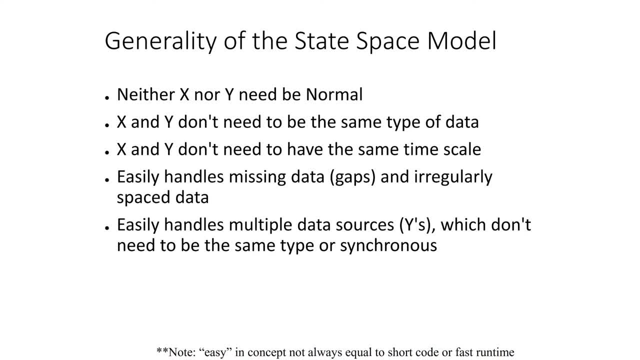 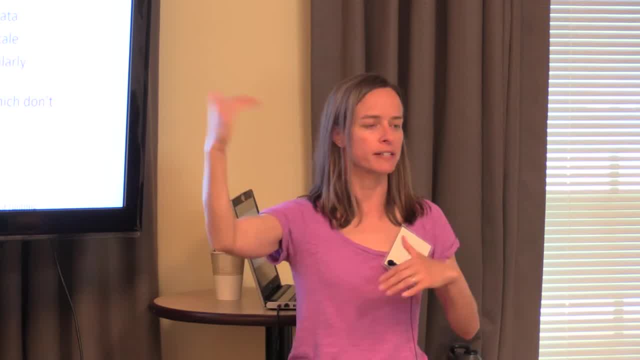 I. you can have multiple types of data, multiple Y's and forming an X. so yet yesterday I showed an example of fecundity that was informed by cones and seeds that were collected at different scales and sometimes in different years. so that's two Y's and forming X. 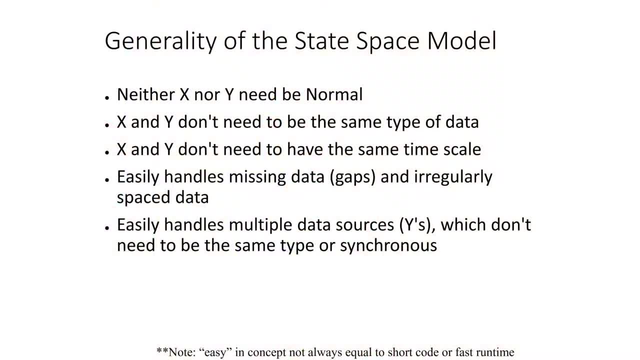 the fecundity there. they don't need to have the same time scale. missing data are fine. again, this is a probability base, so everything unknown, including an N, a and your data set is treated as a random variable right and it'll be drawn from that, that data model and and it handles multiple data sources, so it's a. 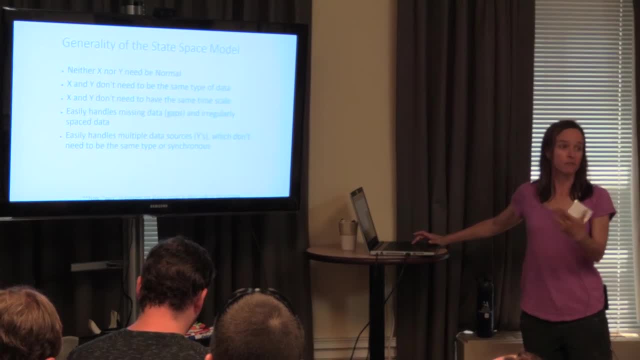 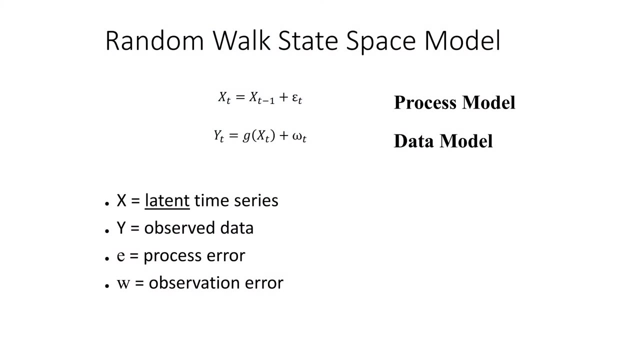 really powerful, inflexible framework for forecasting and for ecological inference more broadly. what we've been talking about up till now is process, where, knowing the last state, t-1 tells you everything you need to know about the current state, plus error. right, so it's a random walk. 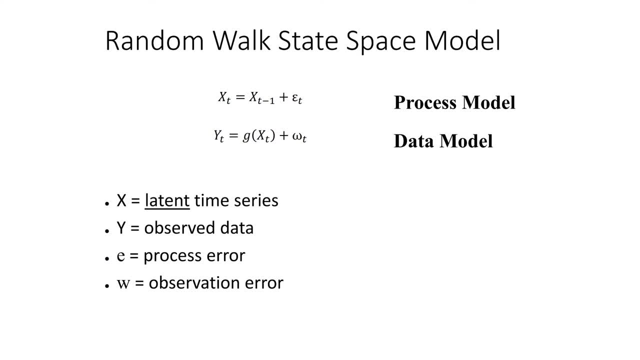 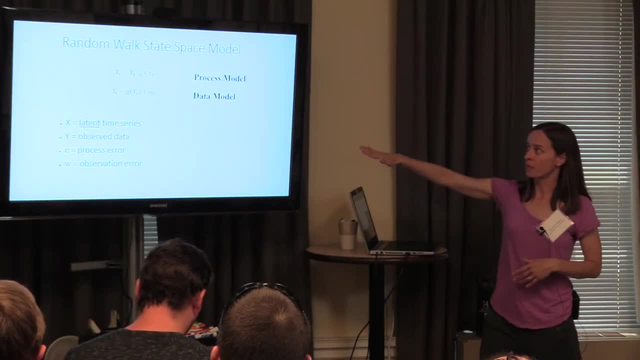 you're. you're basically adding a little error each time to kind of move away from what you were the last time, right, and so that's the same thing I I showed before, but now I've specified that this is a random walk model and you'll hell. 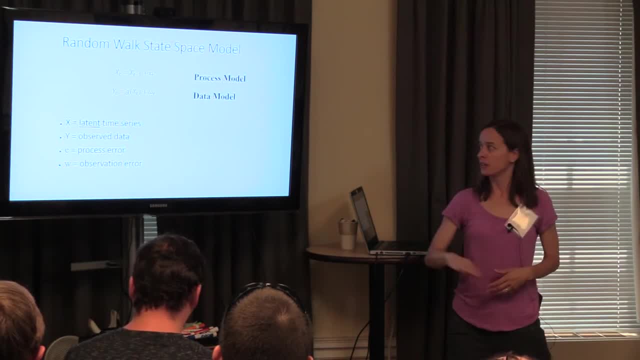 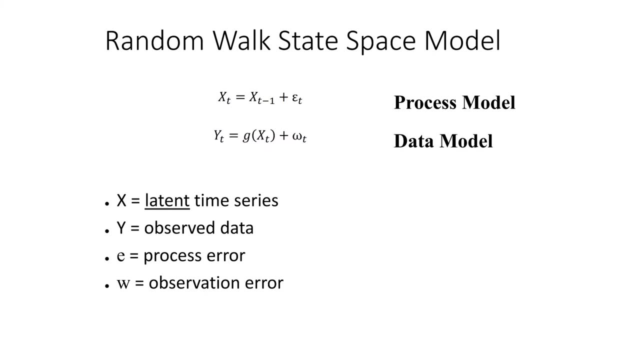 there- that term come up a lot. it's used as a null model. you know, this model tells us that there's no, there's no predictor variables in here, right, so there's no kind of explanatory process, it's a null model that sometimes does better than your best hypothetical explanatory process, but kind of in the 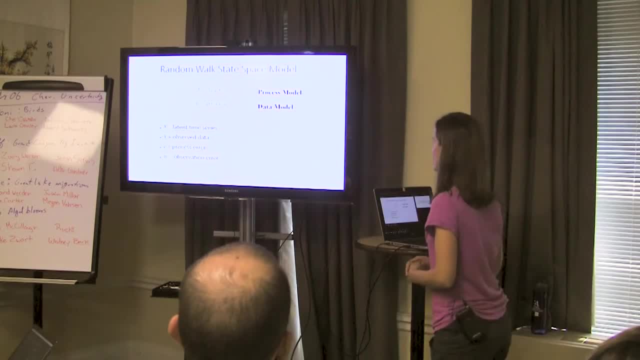 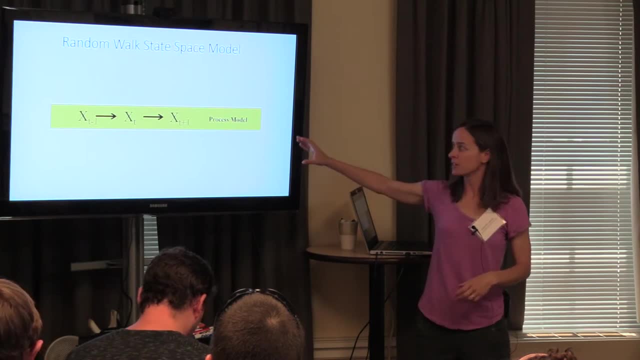 gut, really shouldn't if you got the explanatory process better. so this is often where you start, right, you want to get this working first and again. to break this apart again, in the graphic notation we've got these X's. these are process model. this is the true state, not what we're actually observing, but the 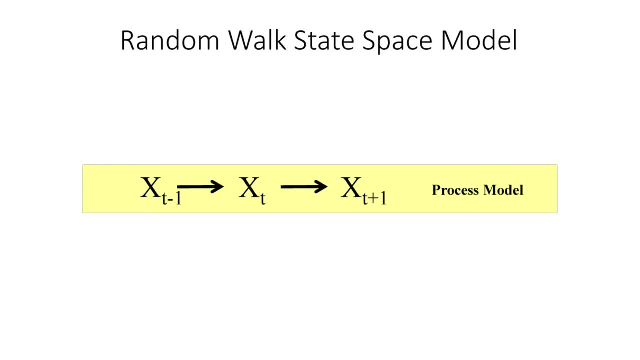 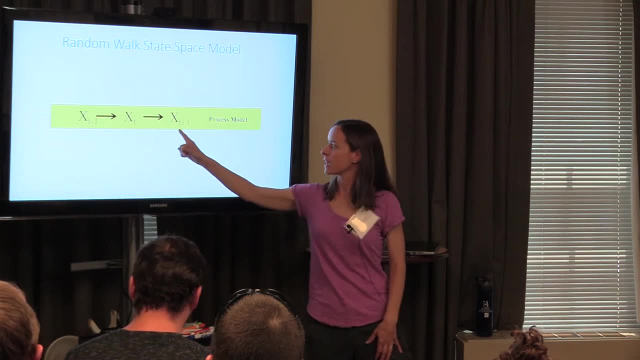 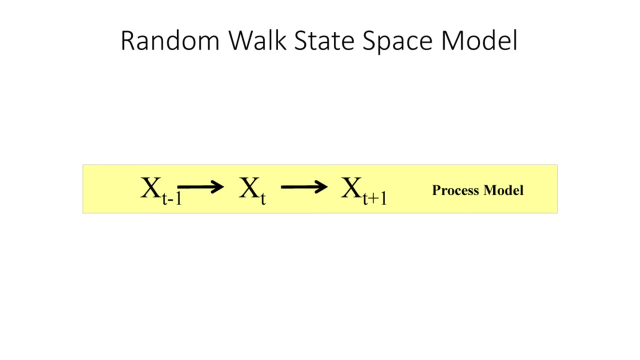 true state. in the example I did yesterday, this would be fecundity. so this is like the: the actual fecundity of a tree at the last time, the current time and the next time. okay, you know. there's no more explanatory variables in this process, it's just knowing. it tells you what it will be. we have a parameter. 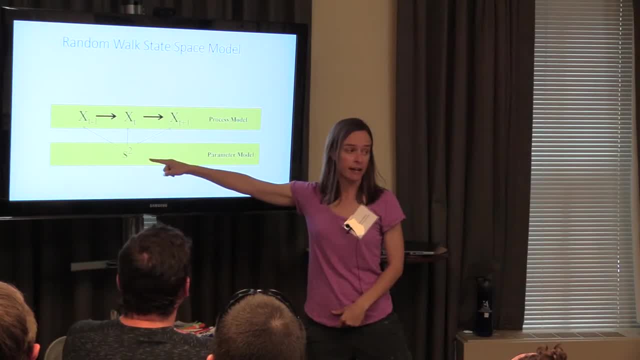 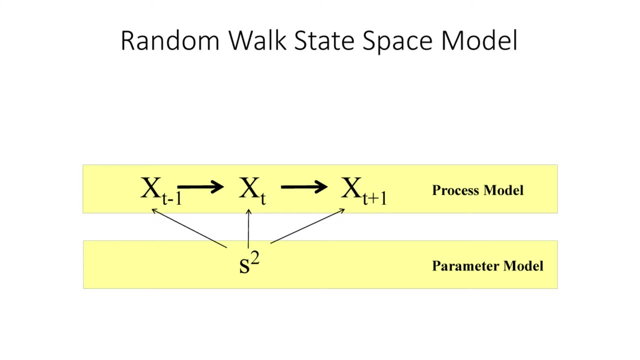 model and and you have some error that you specify and fit on that process and that's how you get to the next time, right? so each time you know where you are, there's a little error, that's added and that's how you get to the next time. and 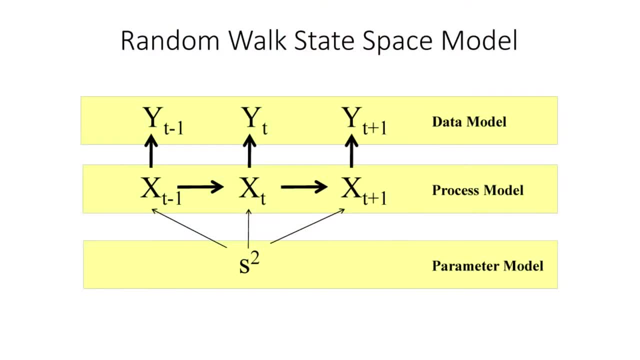 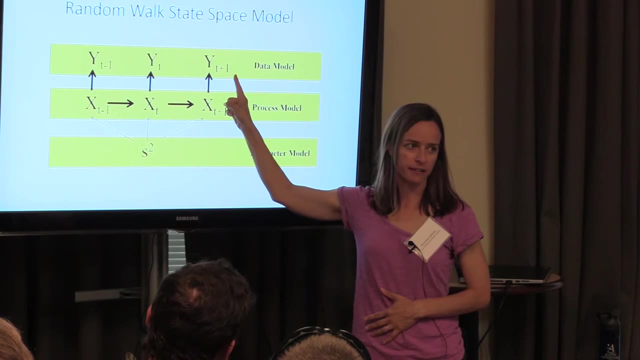 there's no real structure to that error other than what you specify and the data model. these are what you observe and so, importantly, what I want you to get from this kind of slow, tedious process of building this graphic notation is that these are dependent on each other and these are not. these are Y's, are. 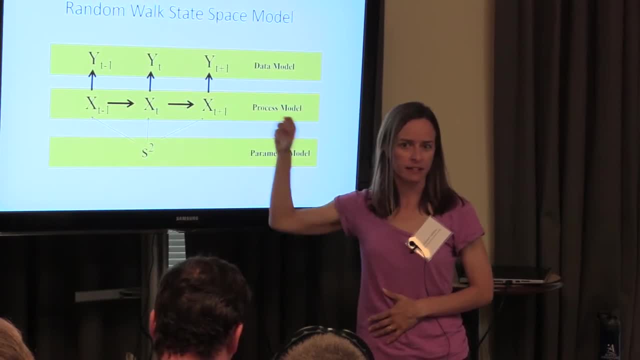 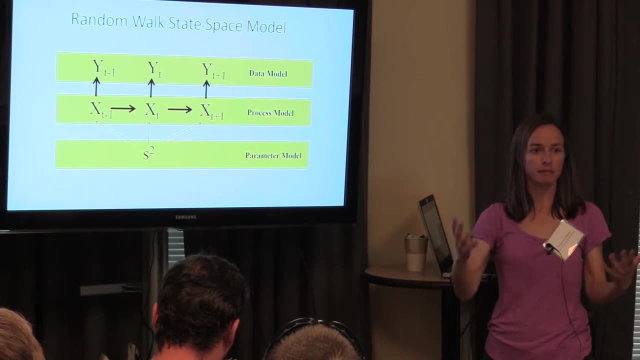 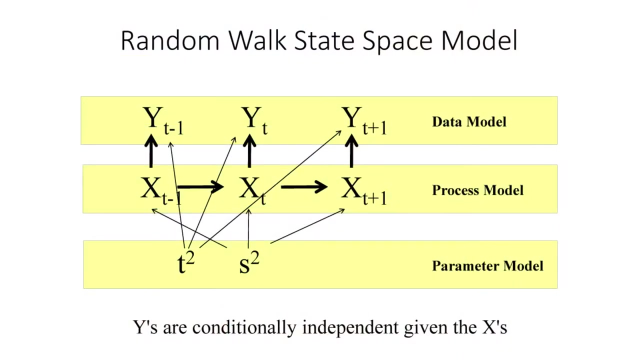 independent, conditioned on the process in X. okay, so which is everyone should go? ah, it's a big deal, right? because, because you've got away from independent, so that's you know we're the error in the data model does not is not beholden to the independence assumption you put your. 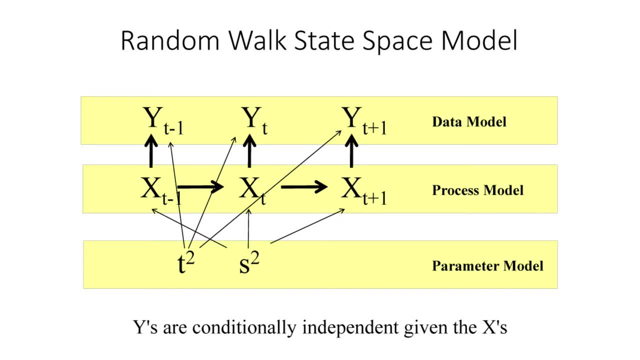 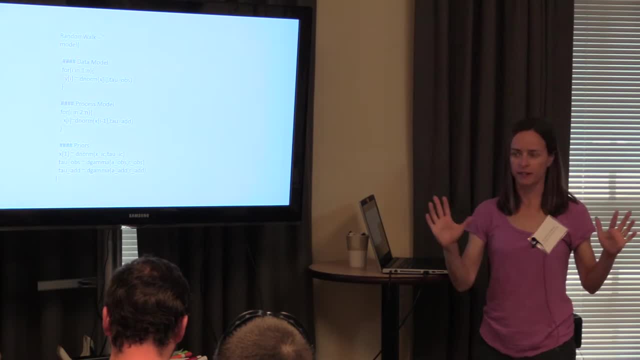 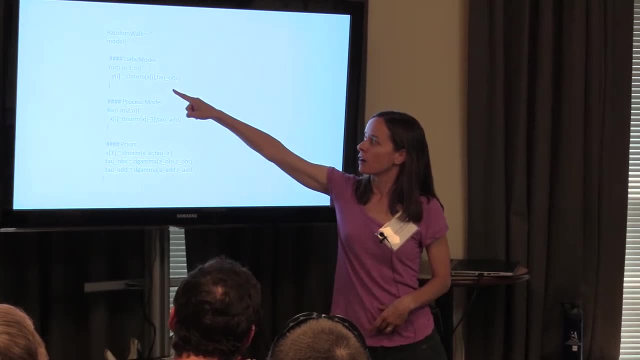 error on those Y's as well. right, but it's not beholden to independent assumptions. so what does this look like in code? now that you guys have all had some some time with JAGS and the code, you've got your data model, they should look really familiar. you know, your Y eyes are normally 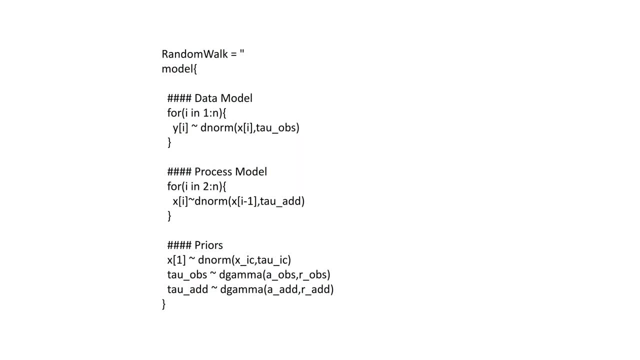 distributed with some mean X. that's your true state, and the true state is normally distributed around the last true state. and then you have your priors, because you're estimating both of the errors: your process error and your observation error. and there's a new line here, your initial, 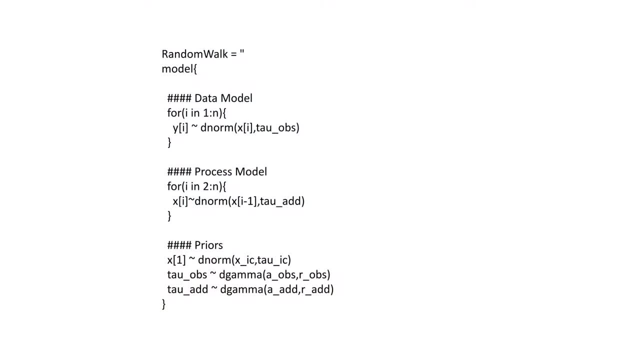 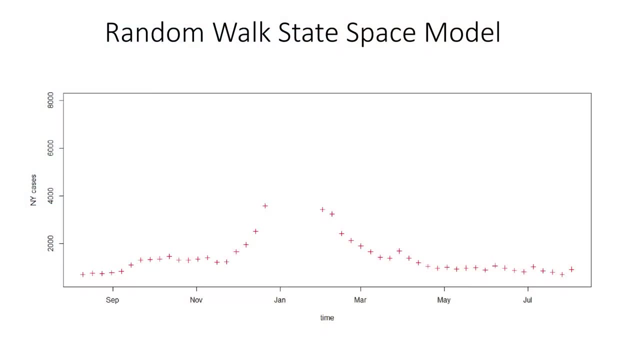 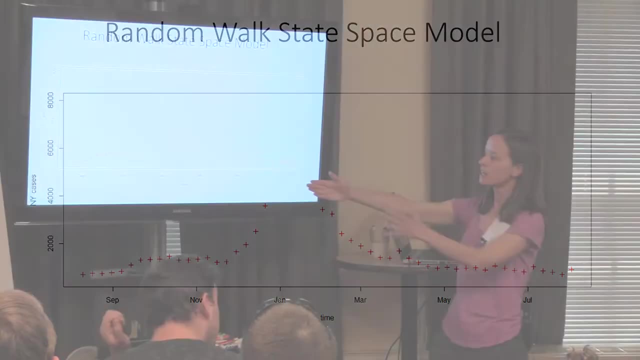 X. yeah, so when you start you don't have an initial X. you need to put a prior on that, your initial condition. these are data that are New York cases of flu from 2015. we've got the months across. the oh, I should have said this is the cases of: 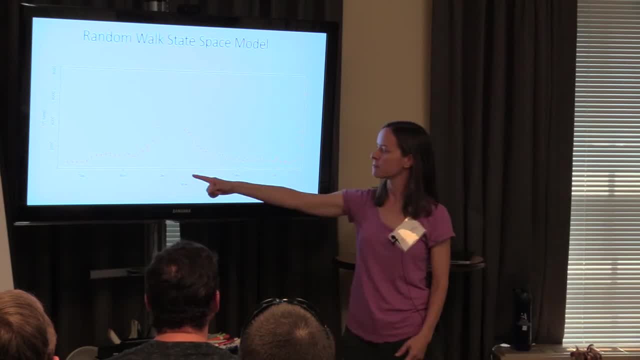 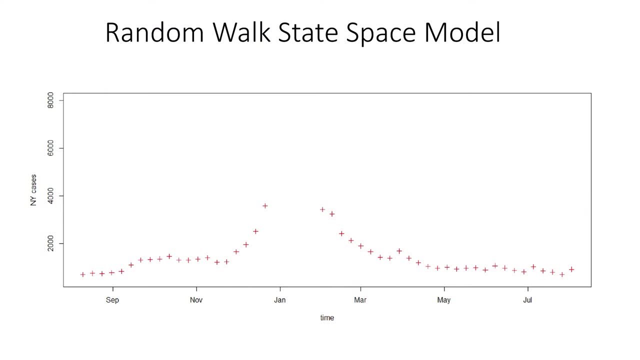 something in New York City in 2015 and the months are across the x-axis and what kind of epidemic happens at this scale. but so it's flu and and there's a missing data here and they're kind of important missing data, right, because you can imagine if 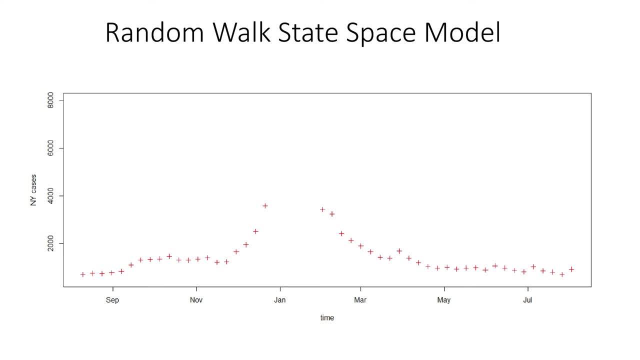 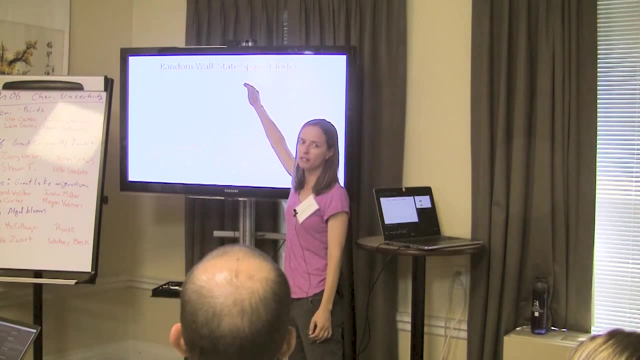 you're dealing with in the public health department, or if you work in a hospital or selling Kleenex. is you know? you kind of want to know, is this gonna like? is this peaked out? am I gonna sell a ton more Kleenex? should I stock the shelves? 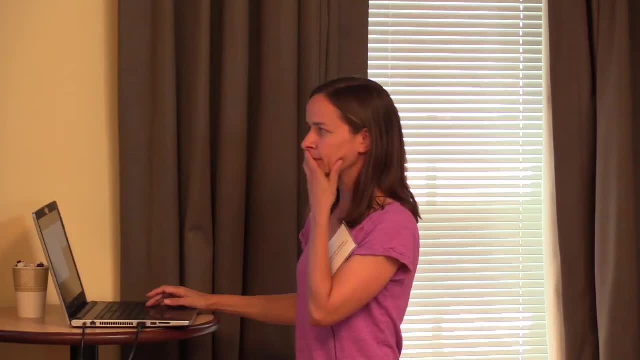 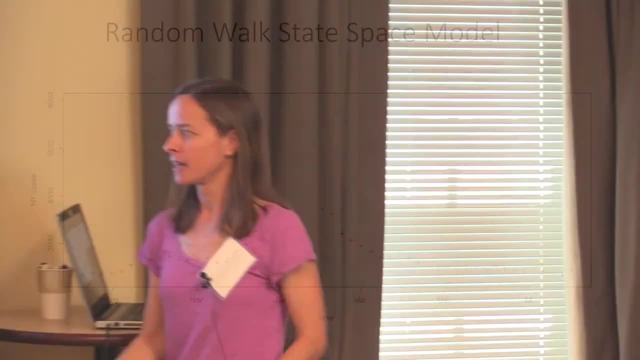 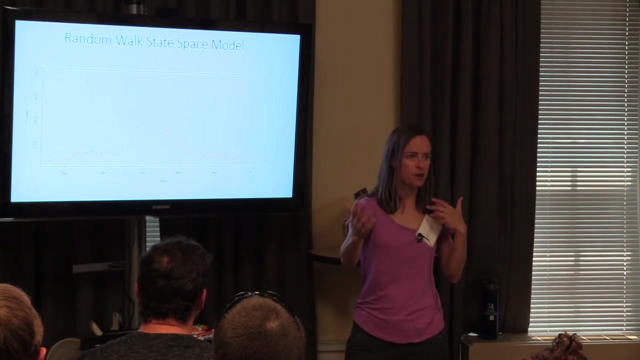 there are reasons that that knowing these data are important. it's obviously nonlinear, right, and- and it's also so- it's the flu. so one person with the flu gives the flu to. you know two people who give the flu to four people, right, so you know that there's some, some structure in the 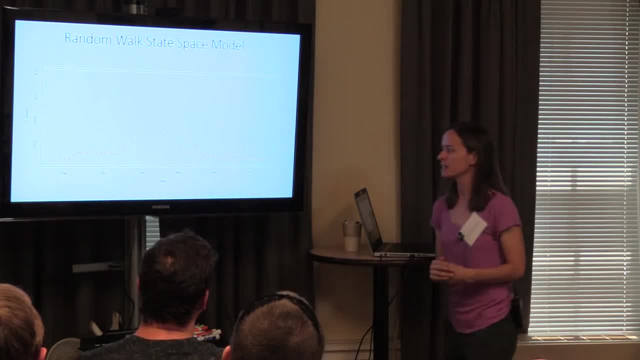 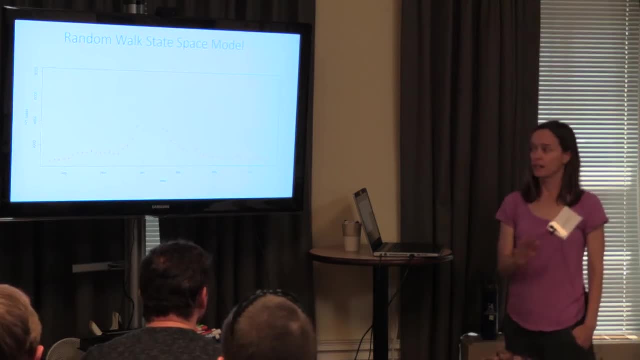 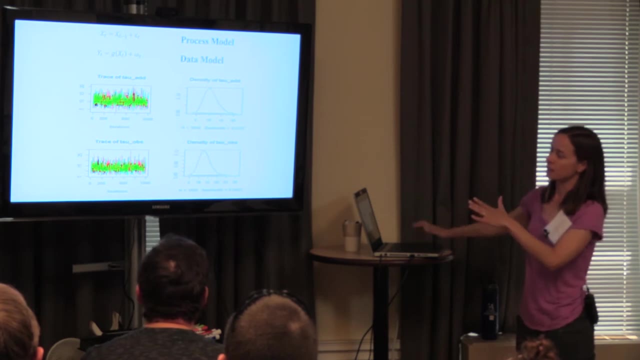 actual spread of flu right, so non non independent cases. so obviously we're not going to fit a line through these, these data and and do anything useful. and so state space approach, and so I ran the state space model on that, the the random walk, and in this case it did a pretty. 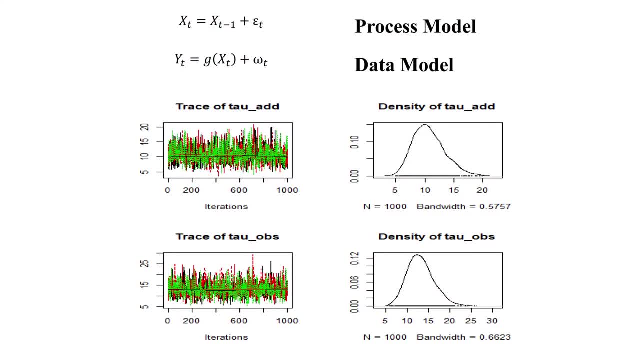 decent job coming up with converged process and observation error. there's a lot of data here, but this is one of the things, so it it's. one of the strengths of a state space model is that you can partition, observation and process error, but it can also be really difficult to partition, observation error and process. 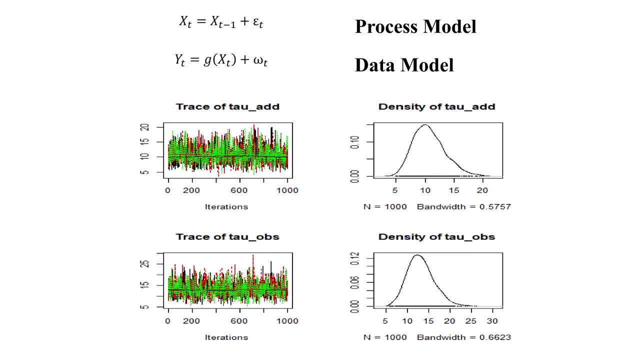 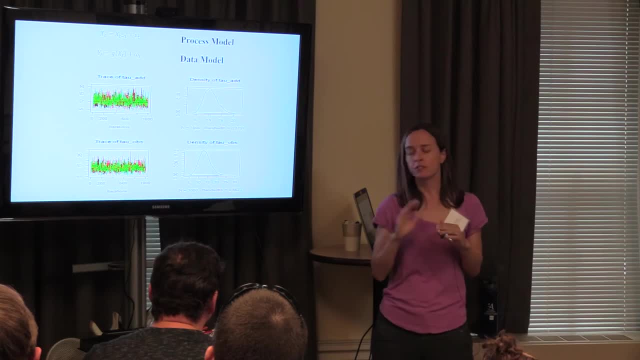 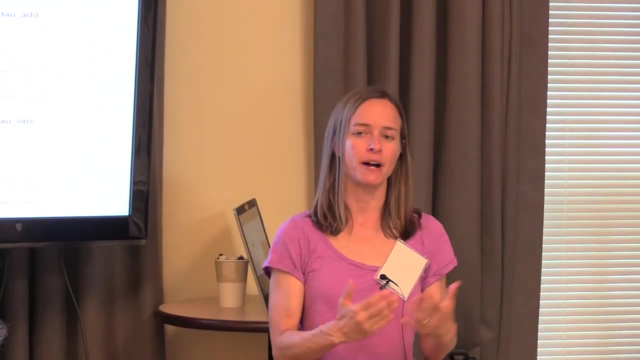 error you can get real trade-offs among the two you know and you could. you could see some kind of bivariate densities come out. you in general, if you have any way to constrain- usually observation error, if you know something about how off you might be and you can. 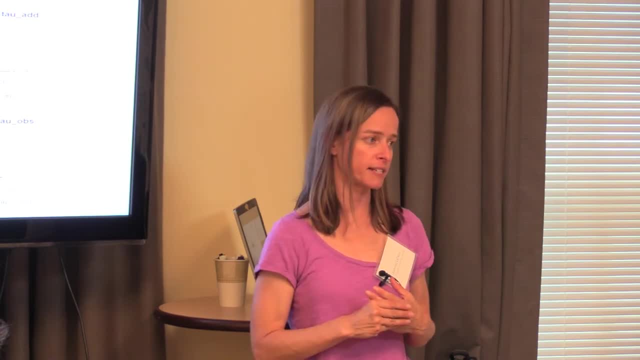 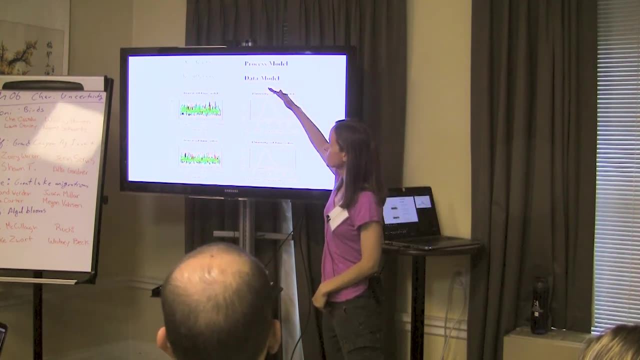 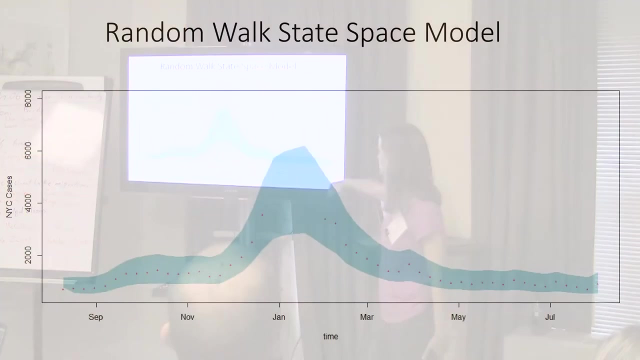 constrain observation error, then you can get a better estimate of process error. and so this is the, so, this. you know the. the random walk was run and things converged, yay, and then you make the credible intervals around that. so these are the ninety-five percent credible intervals you know, unsurprisingly, you. 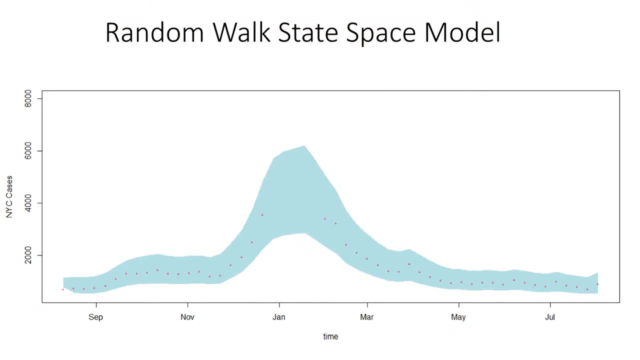 didn't do a great job at the at the initial state, did an okay job at the late state, and you have the biggest uncertainty where you don't have data and in fact, that uncertainty gets bigger the further away you are from data. right, if you remember the, the graphic notation, best information, the best estimates. 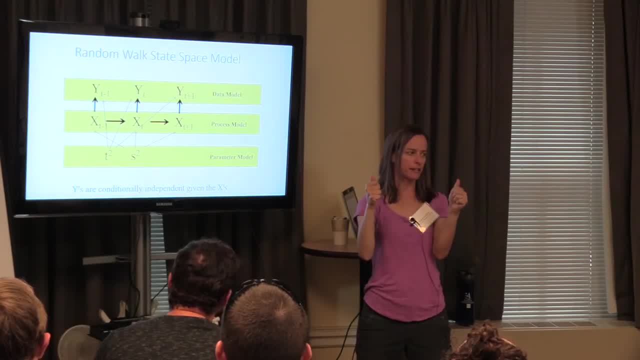 you're going to get about XT are always going to be where you have T plus 1 and T minus 1. if you don't have either of those, then you're going to get less and less certain about X, T, which should make intuitive sense, and so that's what happens here, right, you're. 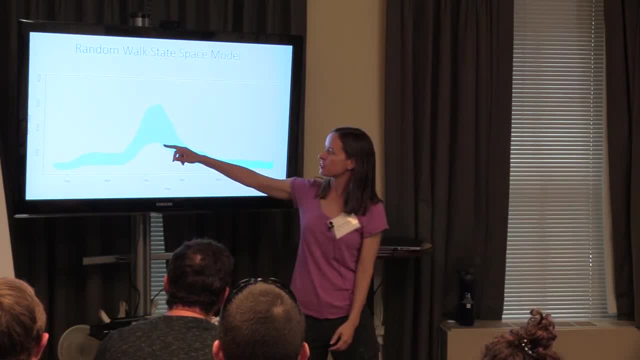 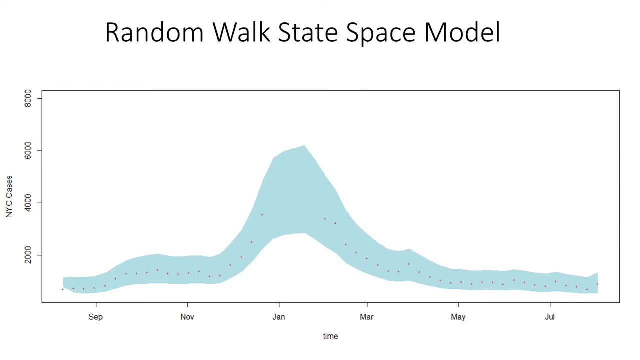 you're not super certain and and you know you get some information- the the flu could peak at 3,000 cases or 6,000 cases. it's kind of what it's telling you and that that's better than no information and it may be less certain. 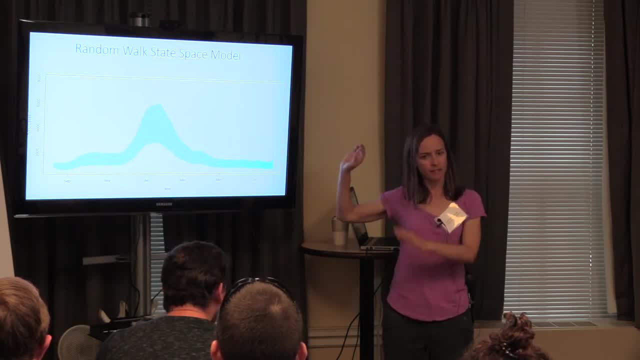 than if I had done the model without characterizing the uncertainty and propagating it. but that doesn't make it wrong, right you're? let you're more likely to actually have the, the true estimate, be within that range, even if it may seem less satisfying to have a. 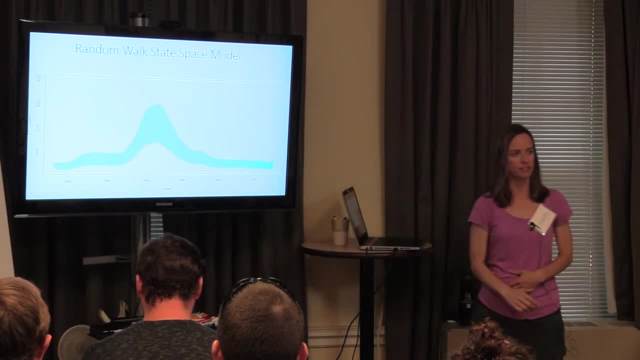 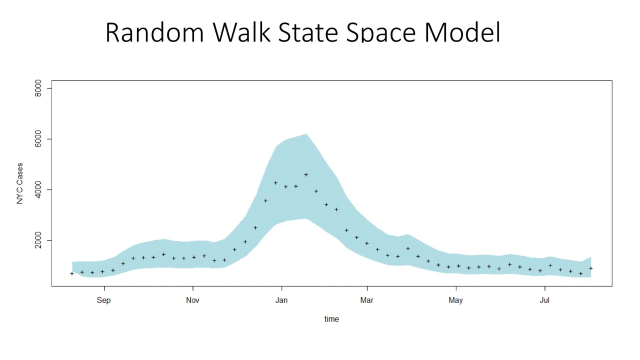 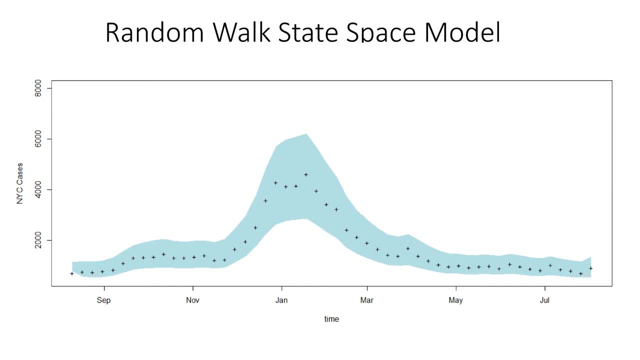 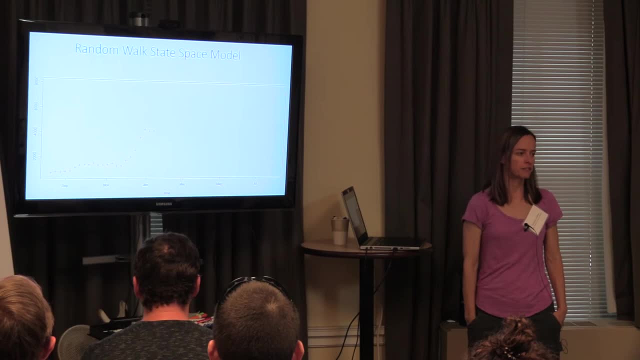 it. so knowing last month's flu turns out to be a pretty good predictor of next month's flu. but what if you only have the first half or you don't even know if it's the first half? what if you only have, like, initial ramp-up of the flu and 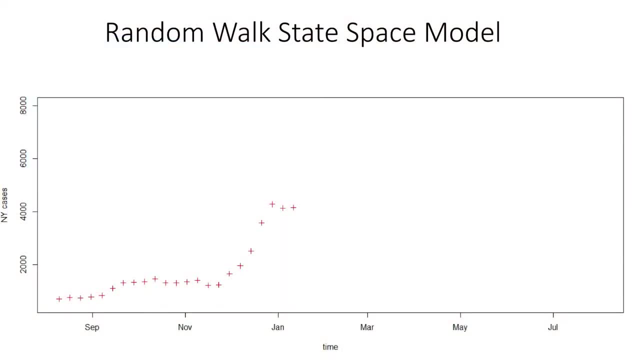 you know you've run out of vaccines and you want to know if maybe you've started to make a difference or if things are actually going to get worse right. so, again, this is an important question and right now you've got lots of data in the t-1 kind of. 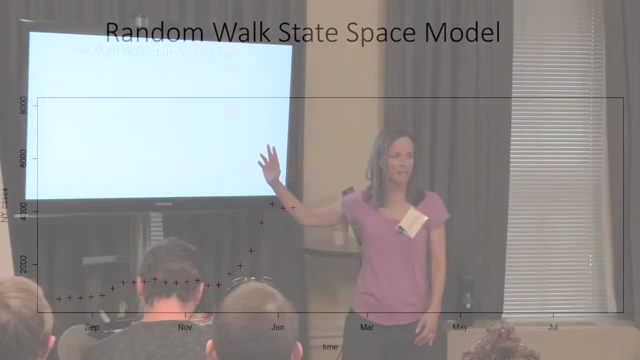 T minus some things you want to that rel, How things will improve through that space. But as you get to the T plus one realm, you're getting into places where you're going to have to be estimating a bunch of Xs with no future information. 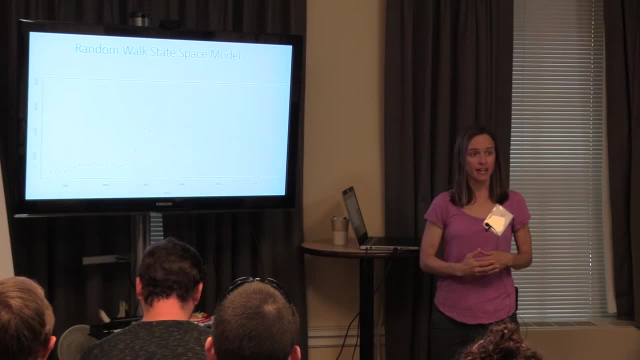 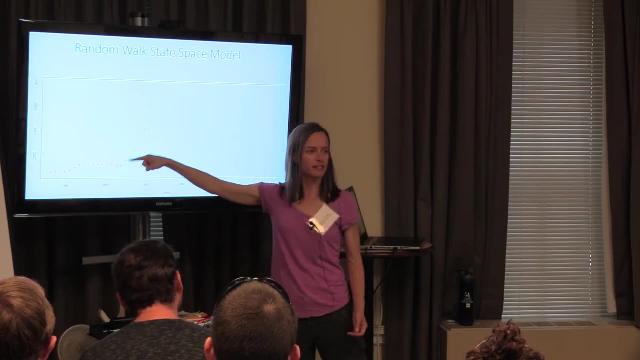 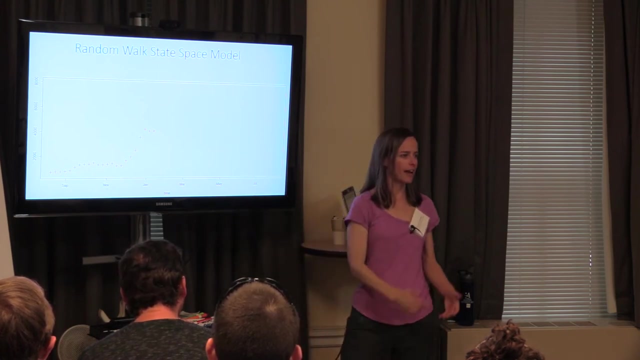 And so, again, you would expect the uncertainty as you get further away from here to get bigger. It doesn't matter if you can fit a spline or something to this perfectly and you just extend it out. you should still get less certain about where you are as you get further away. 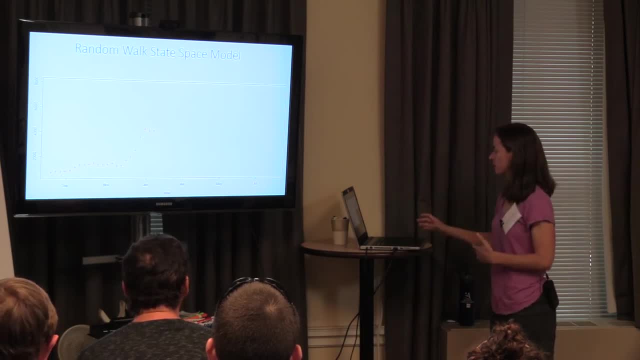 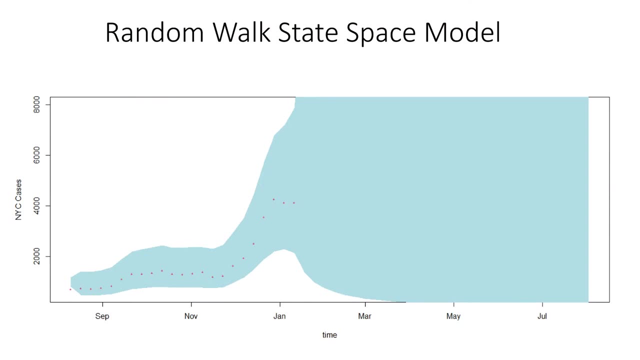 from the last data point you had. So hopefully, intuitively, that should make sense And in fact you can plot that out And even though the first model, where you had some information back here to constrain it again, look like you know, knowing last month is a really you know, powerful way. 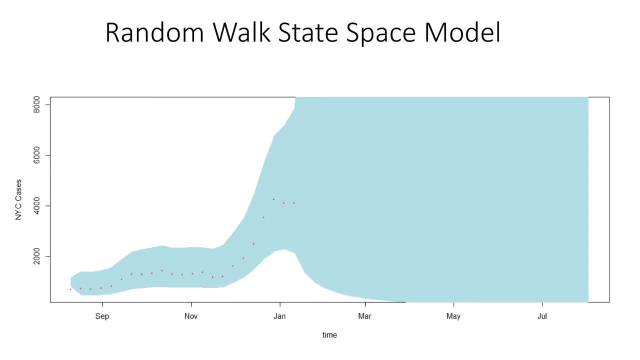 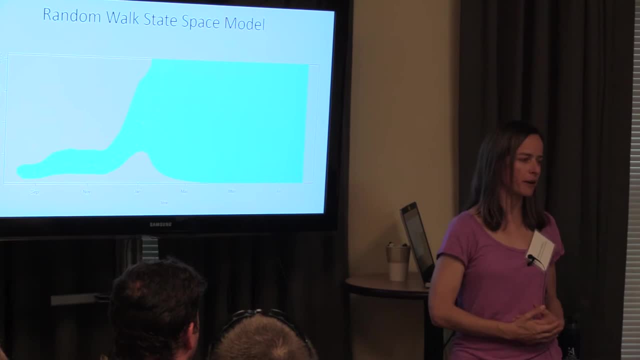 to predict this month. that's only true up to a point, right? So this is good, right, There's more information out there. We're not completely helpless Beyond knowing the current state, as a predictor of the future state. there's got to be more. 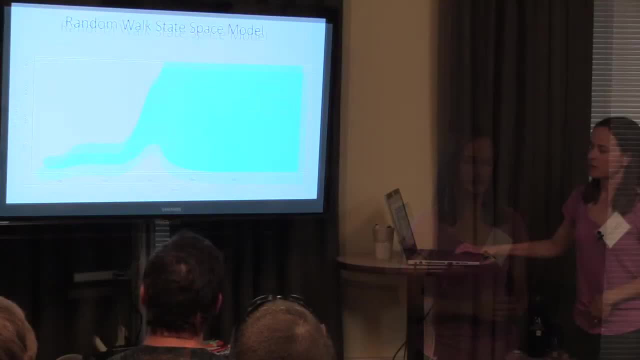 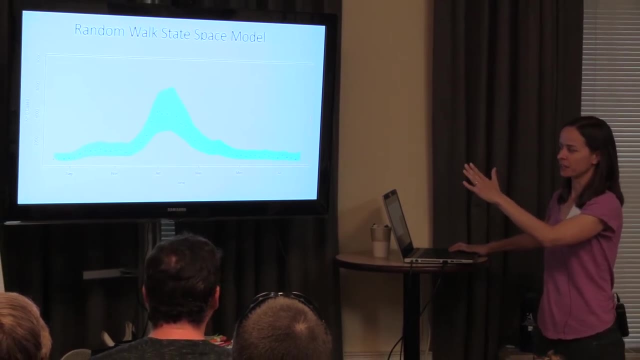 information out there that is important. So this is a random walk right There's and- and even though it looks like it does really good, it only does really good if you have a lot of data. and you have data you know on both sides of the series you're. 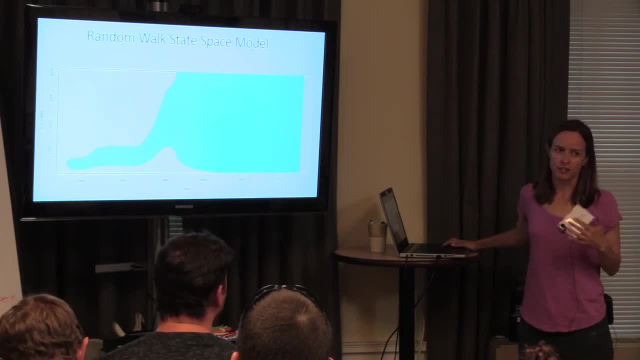 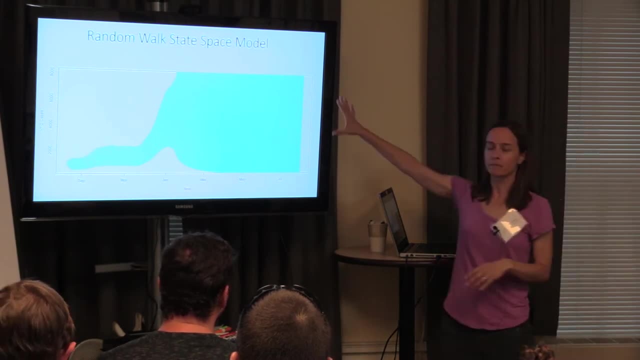 trying to to forecast- And oftentimes we're not trying to forecast things- We already have some future data kind of to bound, And so you know how do we go from boundless possibilities in in the future to to actually 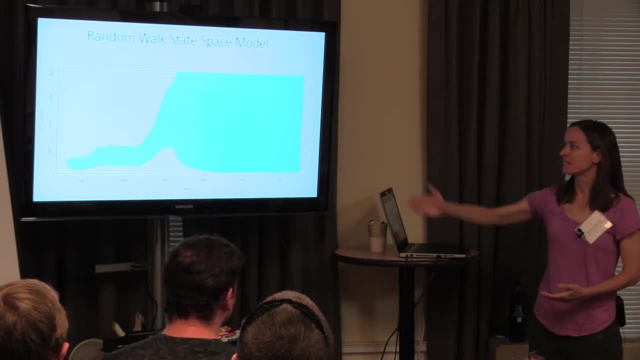 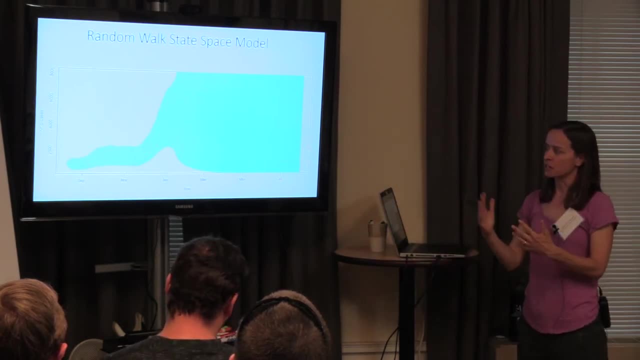 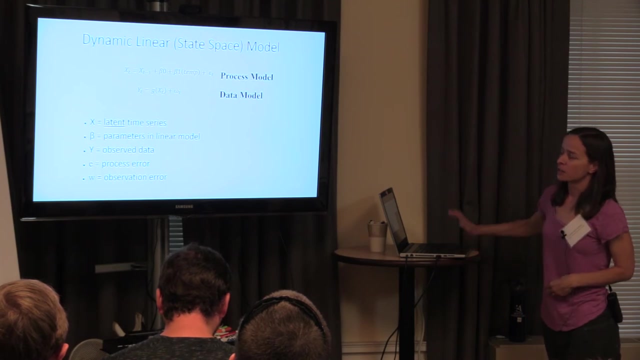 putting some bounds on that, which I mean. this is almost useless, right? This forecast here is almost useless for for management of any sort, And obviously you would want to pull out some predictor variables that that help constrain that beyond the random null model. 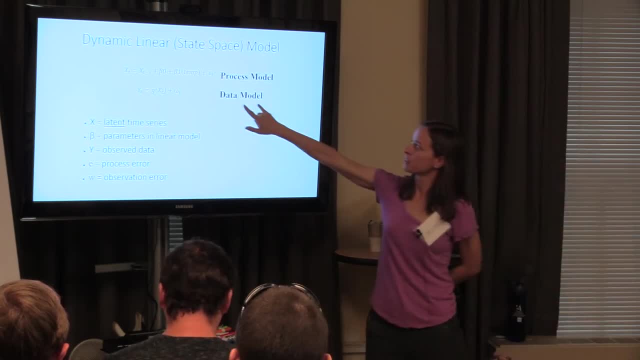 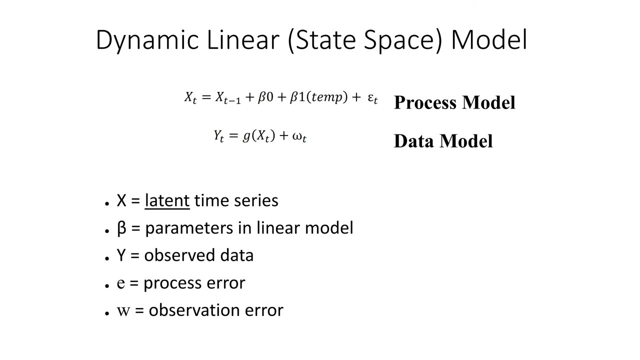 And so a dynamic linear state space model. is You actually just Yeah Kind of add the linear model in right, So that the true state is still a function of the last true state but also of a linear process? And there are many special cases where you move beyond the linear process, and I'll show. 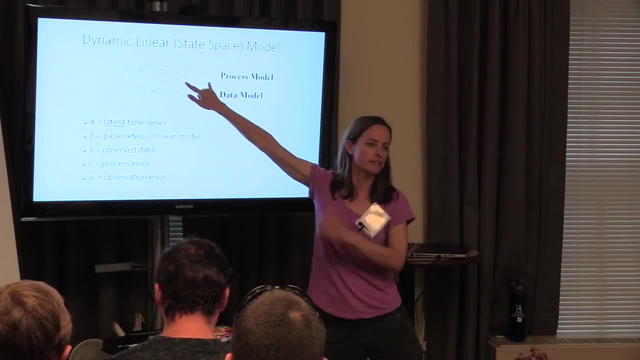 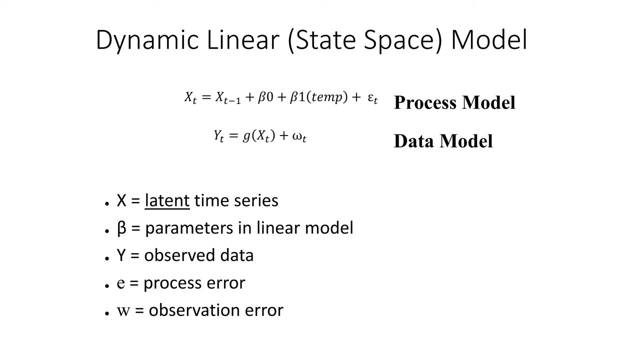 one today, but you've all been doing this And in this case I'm putting temperature in here, which doesn't have. there's some biological reason to think temperature is predictive of flu, but mostly I chose it because things peak in them. 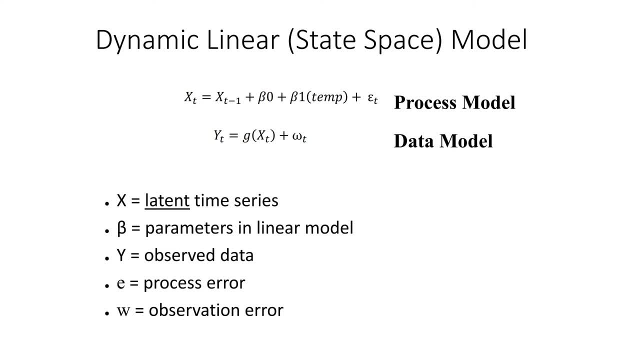 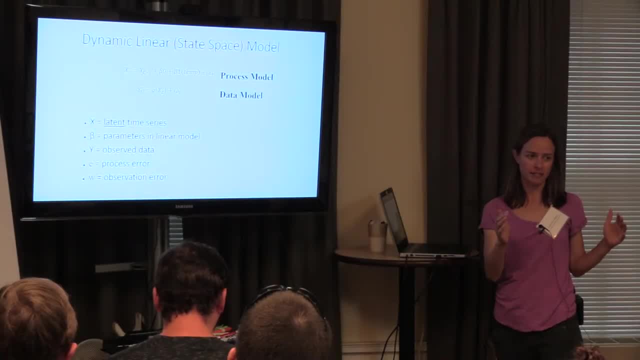 Winter and you and then you still have your data model. I didn't model this, but you can imagine that there were temperatures that were lower in the beginning of the flu season And as they got lower again, the temperature should have some ability to pull that uncertainty. 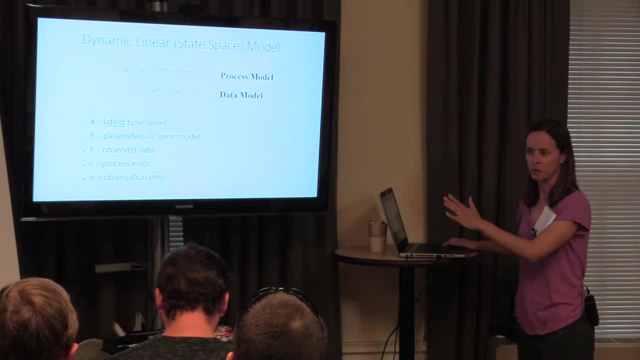 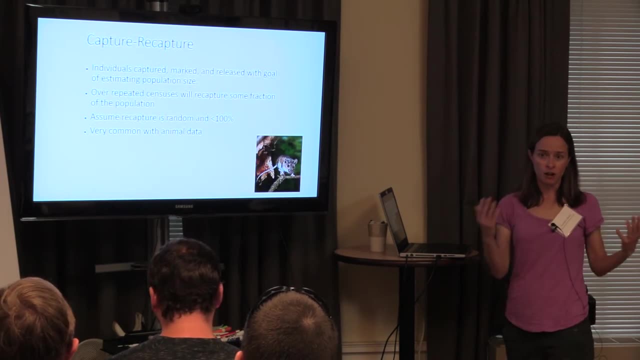 error in Right. Okay, And there are lots of other things you would want to put in if you were doing this for some public health reason. So so you can also do a nonlinear state space in the example I'm going to cover here is kind of a mark recapture example. 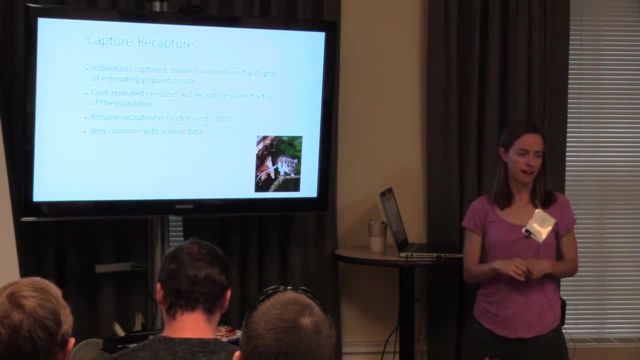 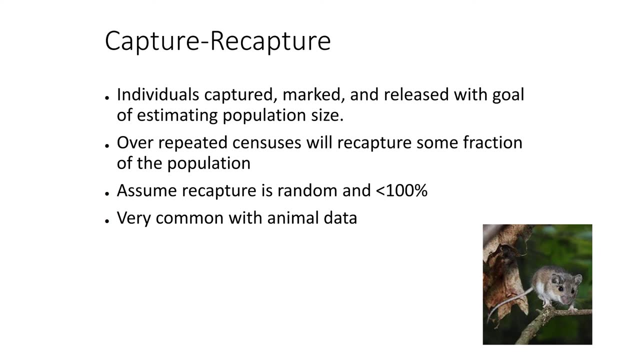 I'm just a lot of people here who think about animals and how you sample animals And in this sampling mechanism you go out and you capture animals and you tag them and then you let them go. You go out again and you capture them again and you assume that the proportion of animals 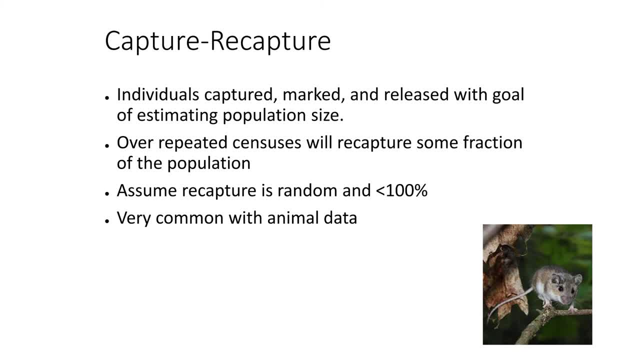 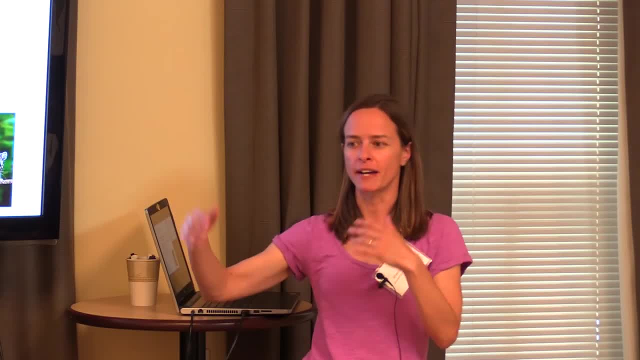 you recapture but you assume that it's some constant, it's some proportion of the total population. right, You marked some proportion the first time and when you go back out and you recapture and you get those marked ones back, that right it's a ratio. 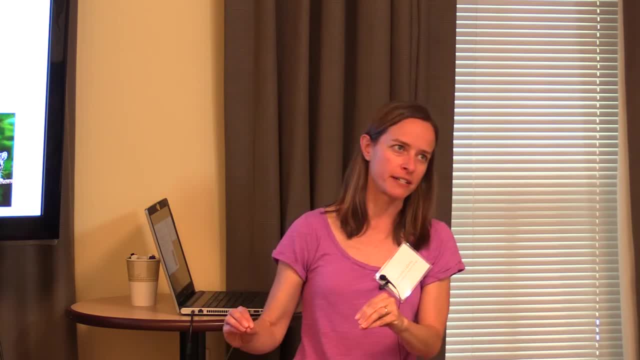 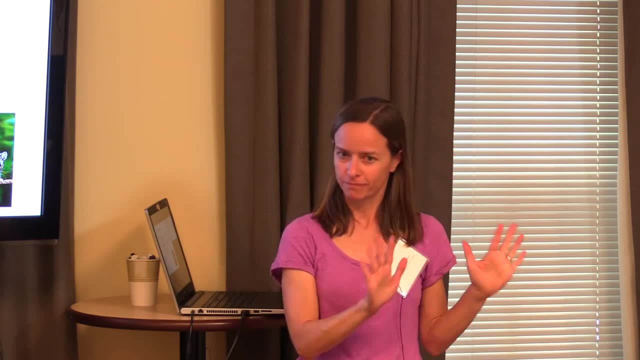 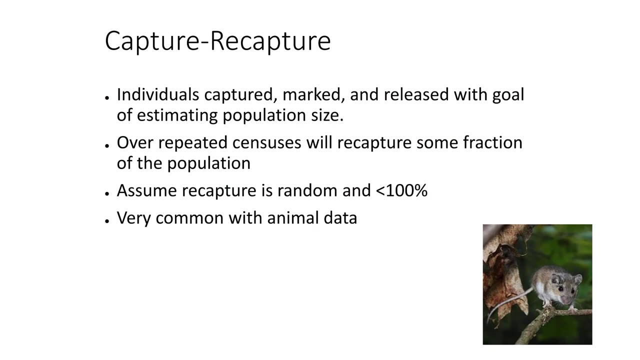 You get. the proportion of marked ones you get, of the ones you marked, is proportional to the proportion of the initial capture and the total population. Okay, So the more you do that, presumably the more information you get. There are some assumptions. it's random and it's not a hundred percent, which usually 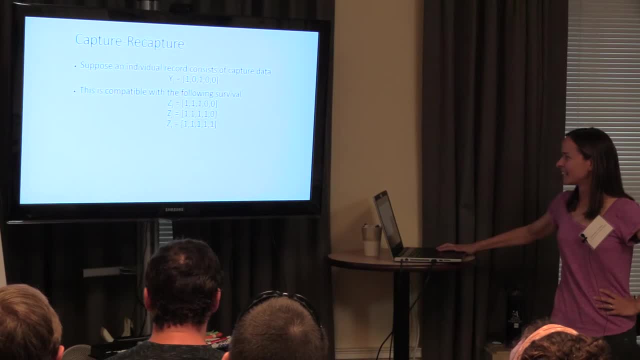 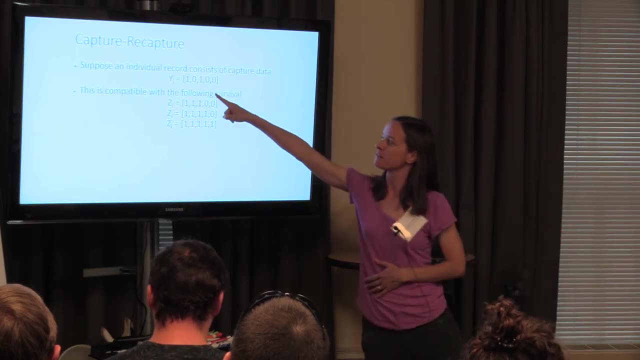 isn't a hard assumption. It's an assumption to meet. Obviously, you don't do it with plants. Okay, So the data look very different than the last flu- counts. So an individual record- the individual is I and the record itself is a vector of in. 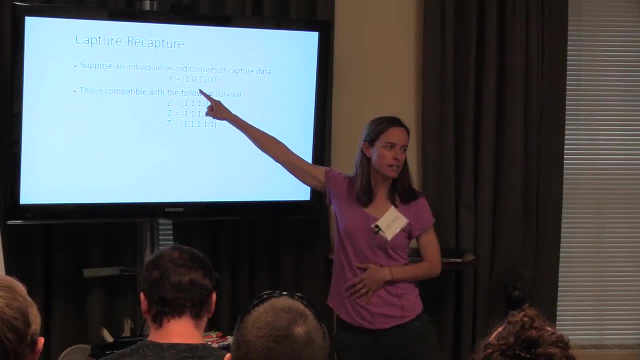 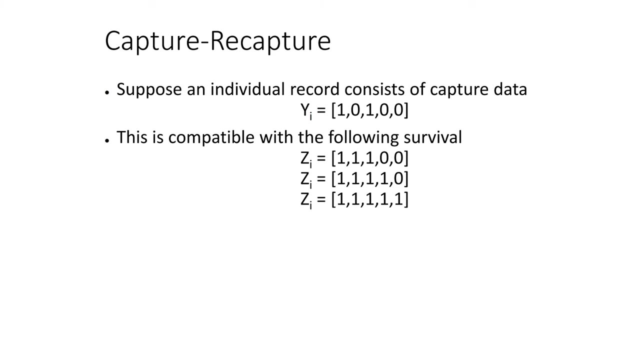 this case, somebody went out five times and they captured it, then they didn't, then they captured it, then they didn't, then they didn't, And so there are different realities that match with this capture history. This is a Y, an observed capture history. 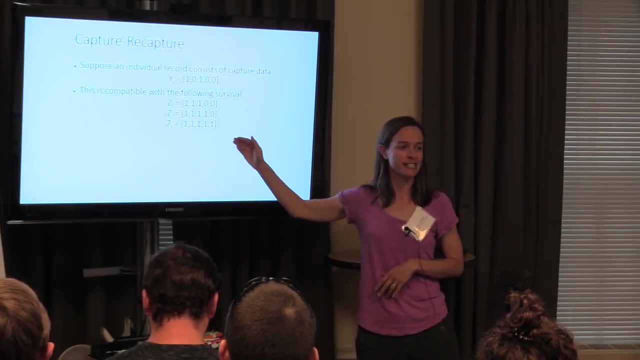 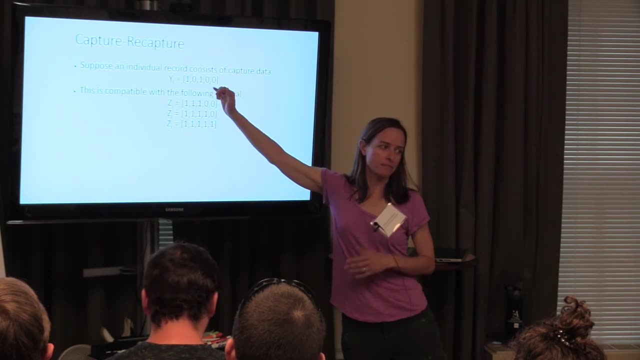 This is, these are the potential true states. So here's Z is the true state, and the potential true states are that it was alive here and and pretty much that's the only one that works there, because then it was alive again, Right. 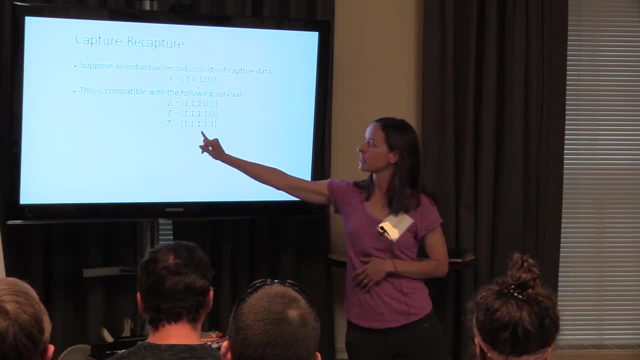 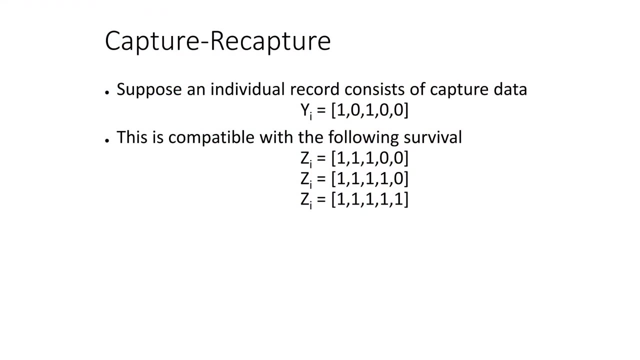 So all of those true states involve being alive but not captured, because then it's captured again And you kind of assume if you capture it- that is unless the the, the way you marked it was in some way vague- If you capture it and it's been marked, it's alive. 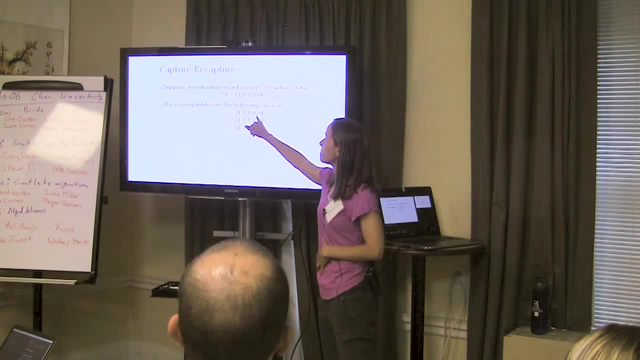 And it survived until you captured it, right By definition. But you don't know about these last two, right? You know that that your capture probability isn't 100%, because you got the zero and then it showed up alive again. 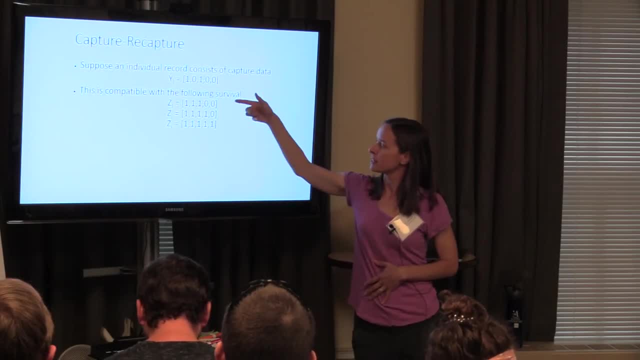 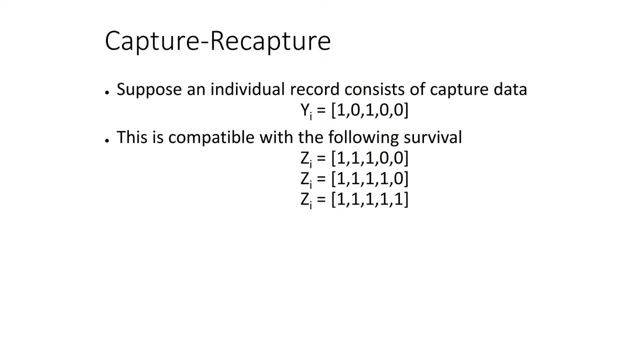 And that actually is good. So you don't know about these two, So you so the. the different possibilities are that it that it died and you didn't capture it, or that it survived one more capture, one more sampling period, or it survived all of. 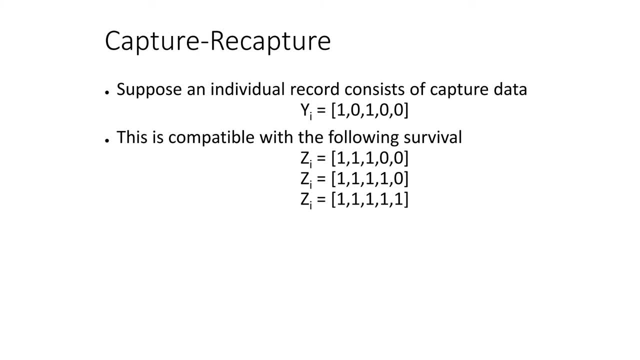 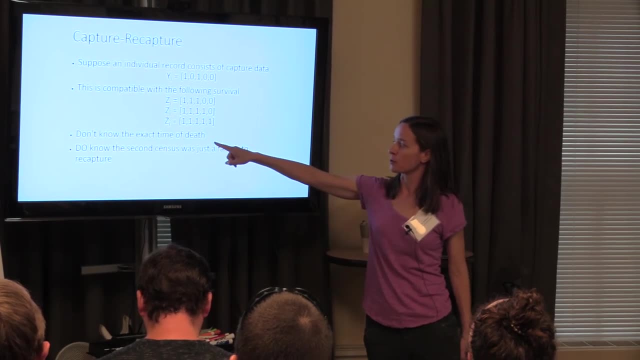 the sampling periods right. And so now we have a a true state That, instead of being a continuous distribution- we're not going to describe it that way- We're actually going to define the discrete possible states and assign them probabilities. From this we we don't know when it died, but we do know that that we didn't capture. 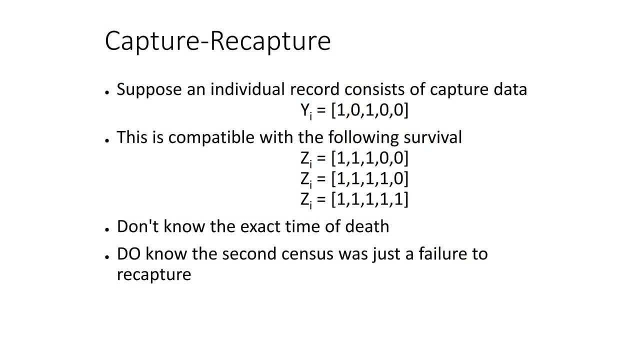 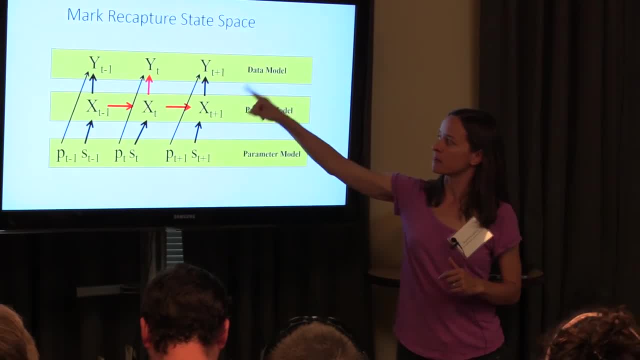 it with 100% probability, And so we get some information about survival without being recaptured. So this is the graphic notation. You've got your, your observations that are independent, right, There's no arrows connecting them. You've got your process model that are dependent through time. 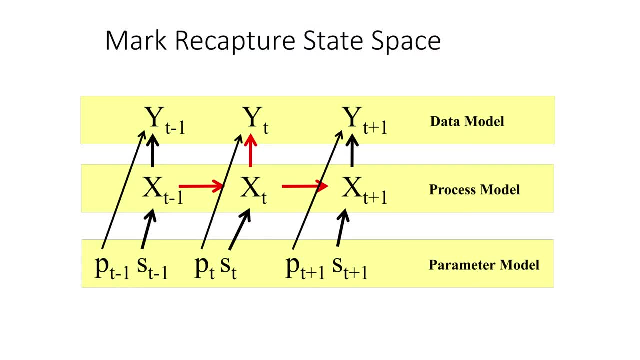 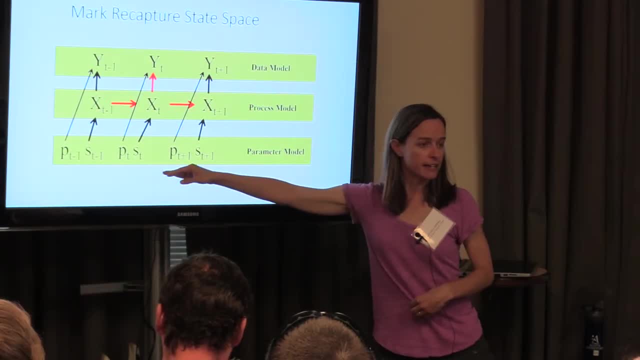 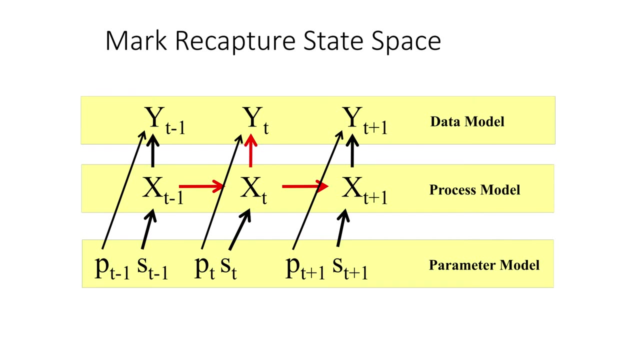 And you've got your. in this case the parameter model is doing error. that also varies temporally. You could just have one P and one S and you could say that all Xs have the same constant variance, or you could imagine that variance might change throughout the season and your. 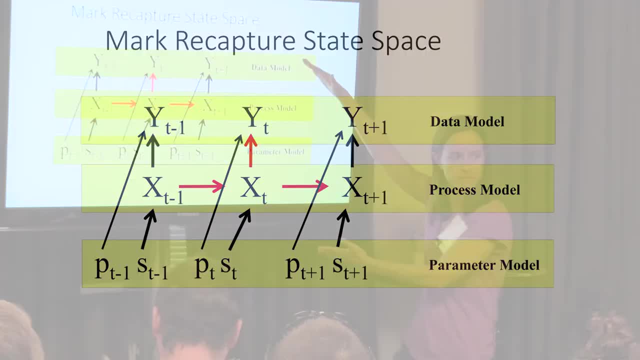 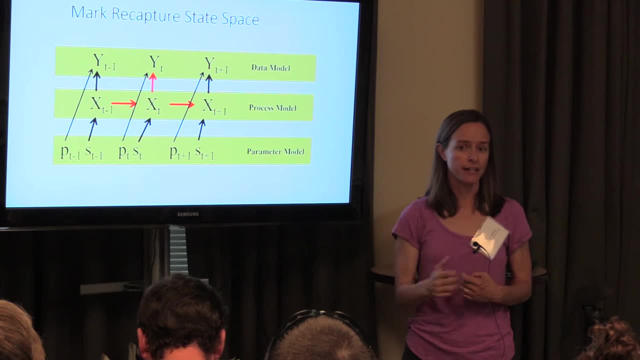 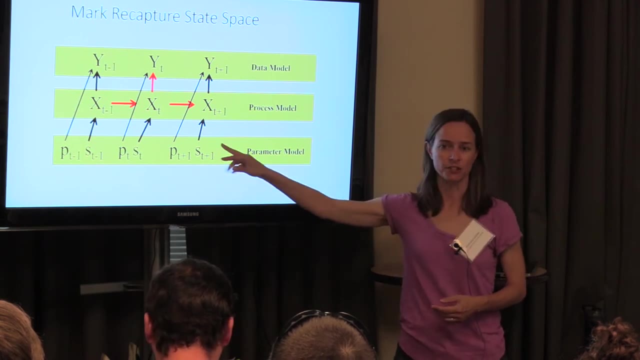 ability to observe might change throughout the season. So, in this kind of example, we're assuming that the variance In our ability to observe, given that it's alive, and our variance in being alive vary during the course of T's during the progression of of these data. 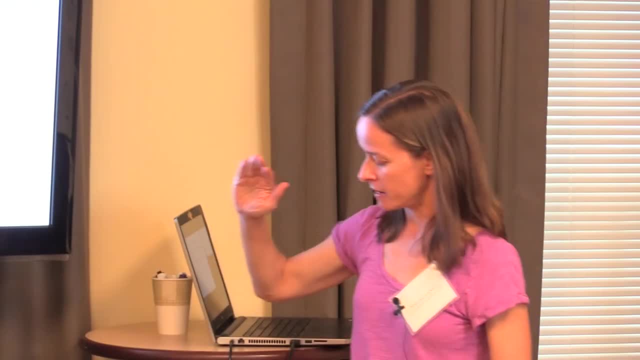 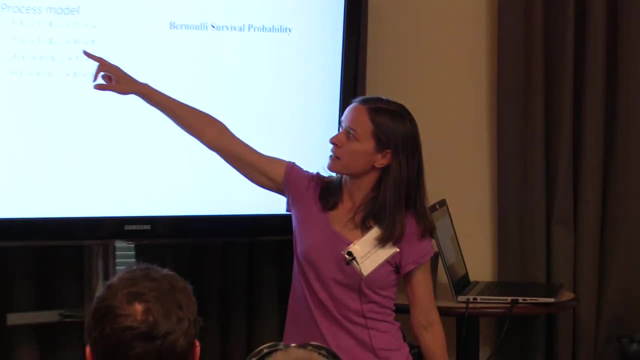 So, survival, we're going to use a Bernoulli probability And in this case again, we're setting up these, these kind of discrete probability descriptions. So you've got the probability that X- the true state at time, right now- is alive. 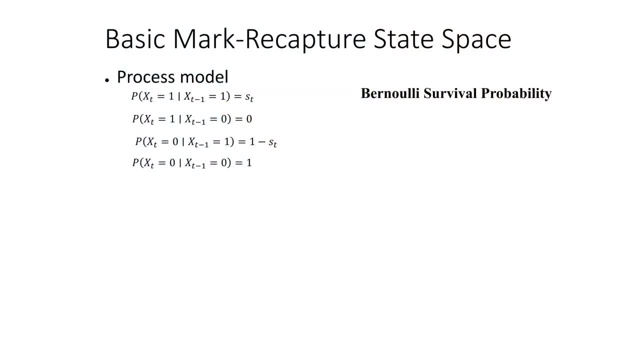 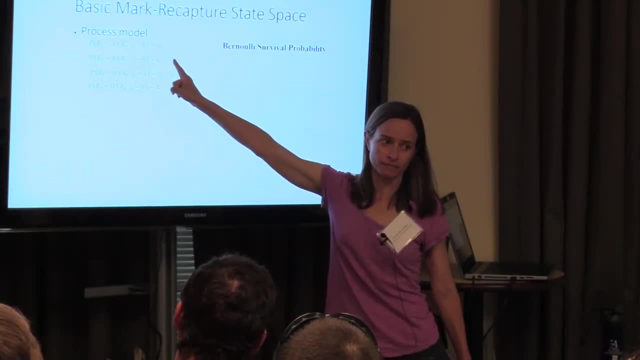 Given that it was alive last time. Okay, So we're defining that as ST and the probability that's alive, given that it was not alive last time, is zero, And then the probability that it's that you don't see it, given that it was alive last. 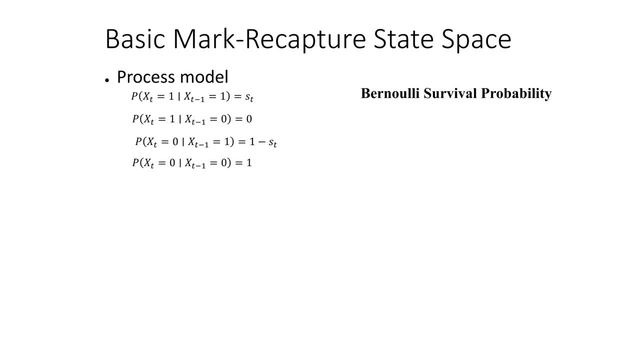 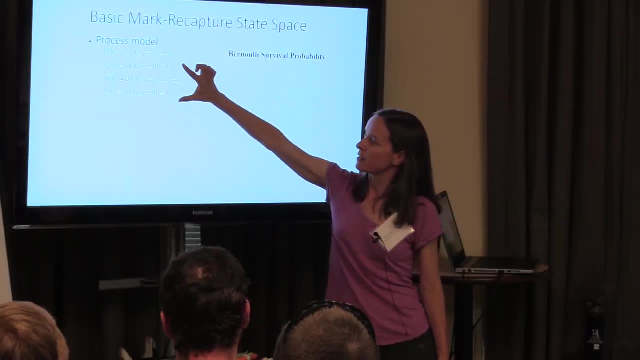 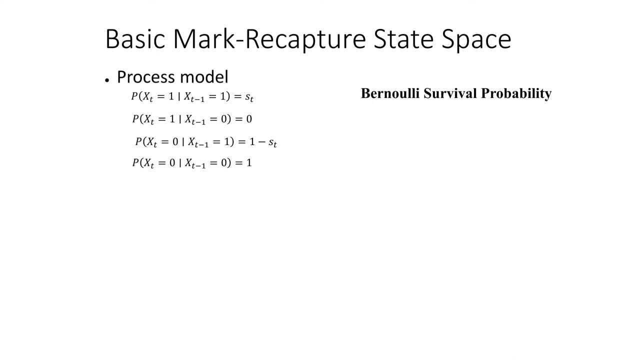 time is just one minus that alternative right. There are two options there, and and and they add up to one. And again, there are two options here: the, given that if it wasn't alive last time, it's either not alive this time or it was alive last time. we already said that's zero. 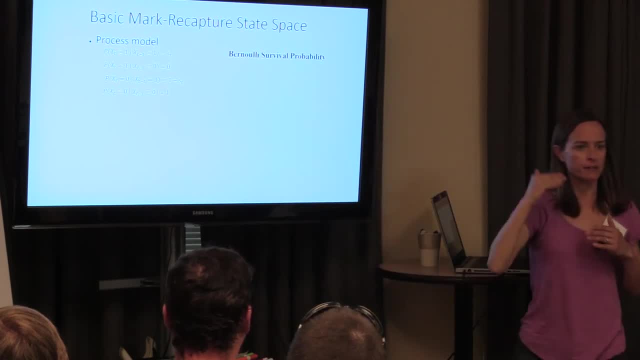 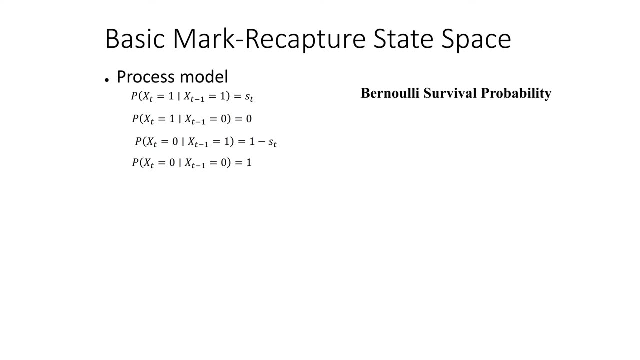 So it's one right. So you've got two different ways that you're getting to a probability of one. The probability of your different states, which are zero and one, each have to equal one because we're in probability realm, So it has to equal one. 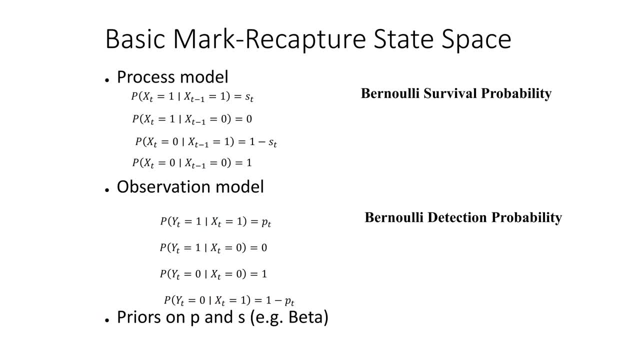 And then you do the same thing with the observation model. But the observation model, remember, is not Y's, aren't dependent on each other, So it's Y, It's not alive condition, or you don't observe it, conditioned on the fact that you you. 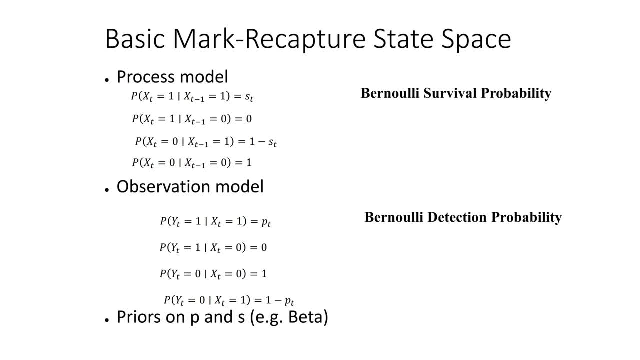 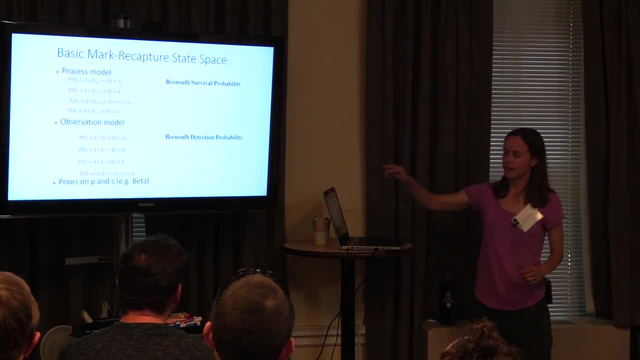 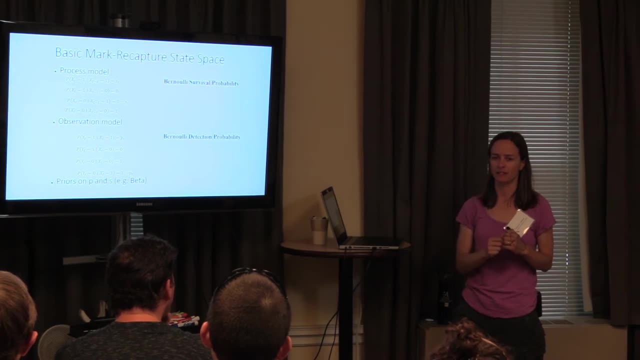 really didn't estimate that it was alive last time. And then you put your priors on the errors in this model And I I guess I will point out that I I've noticed as I've gone through this slide: sometimes I'm using T plus one and T, and sometimes I'm using T and T minus one. 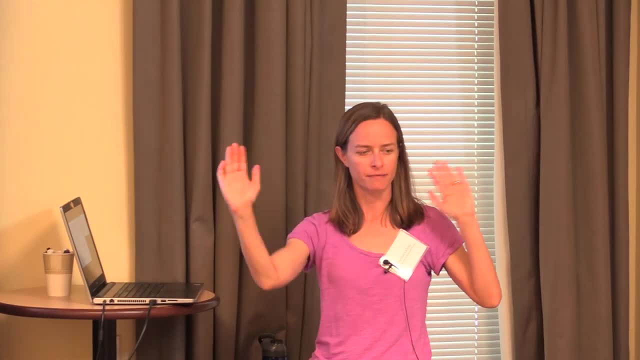 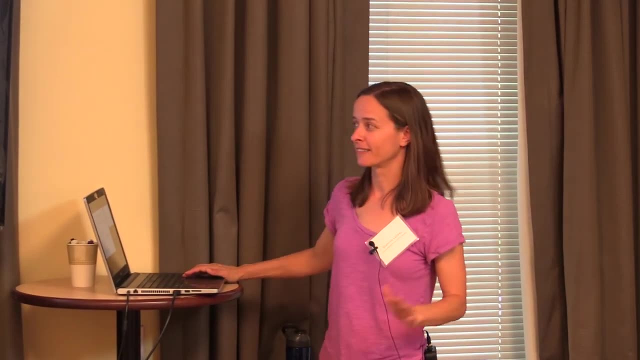 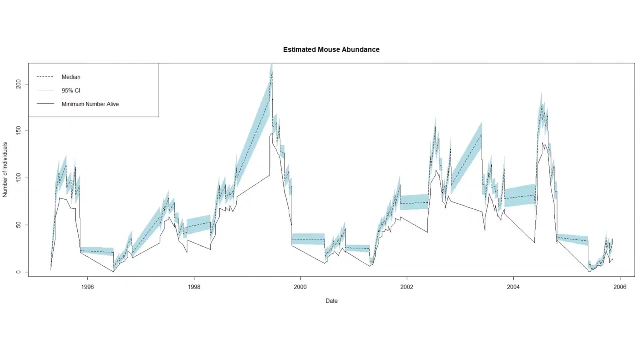 Just remember the graphic notation: where you have X, T is in the middle, and they're both important. So if it wasn't bothering anyone, then forget. I just said it. And so this is actually data from her own, John Foster, who is working on a mouse recapture. 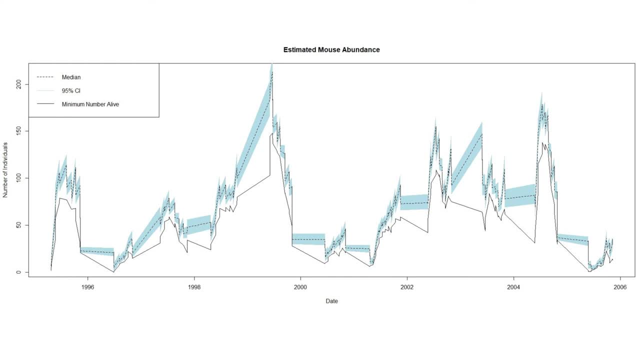 study that that's 11 years, So. so I wanted to have a, a final kind of figure to show that you know, even with this non-linear approach, you, you get very similar, credible intervals and they get wider right. 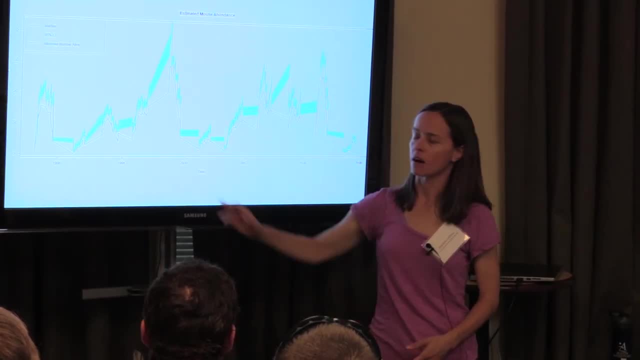 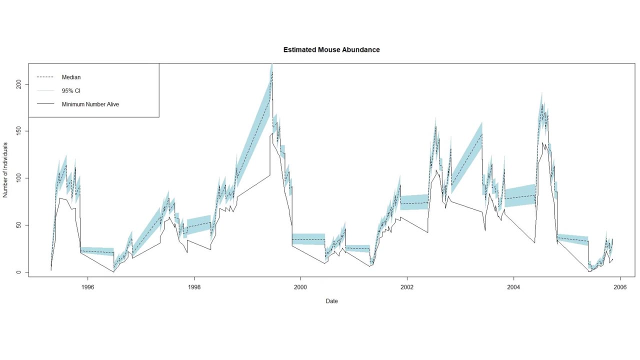 So So you know these parts are. I'm going to put the data on, but those parts are where where there aren't data, and he's estimating this on a daily, you know, are they alive on a given day? 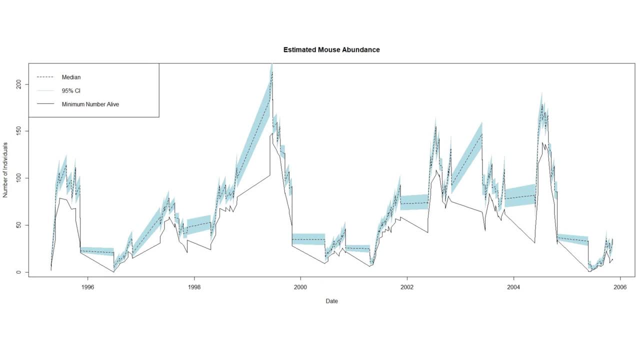 And so there's lots of days often in between sampling bouts, And the longer that goes, the wider the uncertainty gets, which is what you would expect, And- and these solid lines are the minimum number alive. So you know that, that you caught 10, there's at least 10 out there that are alive. 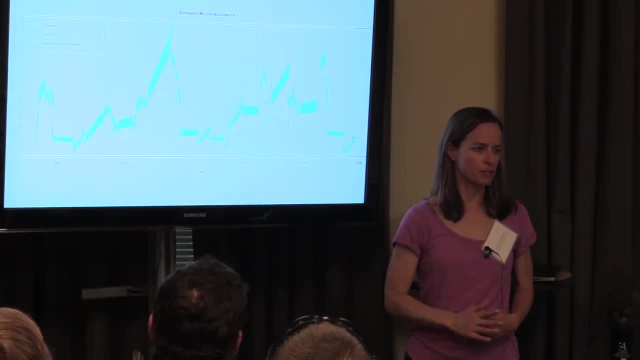 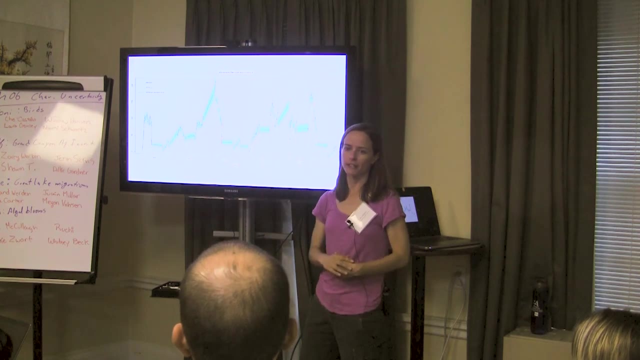 And so we plot that to make sure it's different below that, Yeah, Which would be an indication that we had the dead thing showing up in the trap. Yeah, But it is also just really cool data, so he's doing a good job with it. 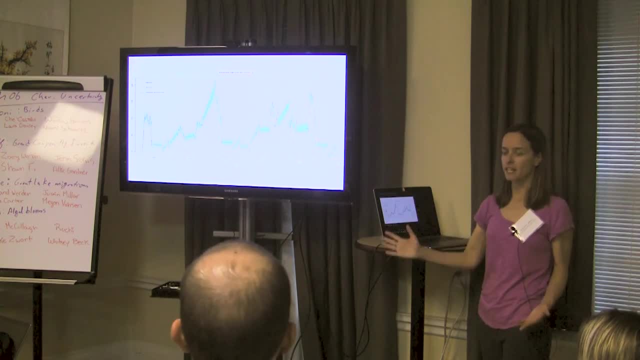 And so that's the end of the kind of introduction to state space that I had prepared.